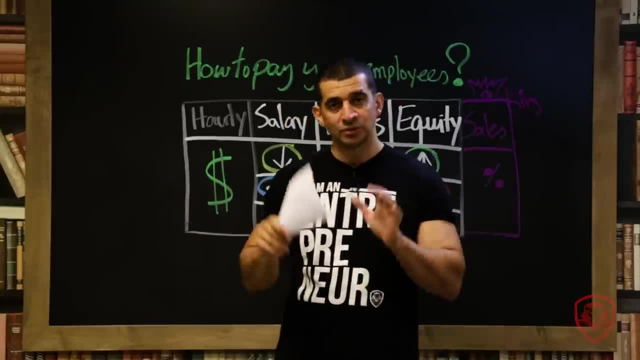 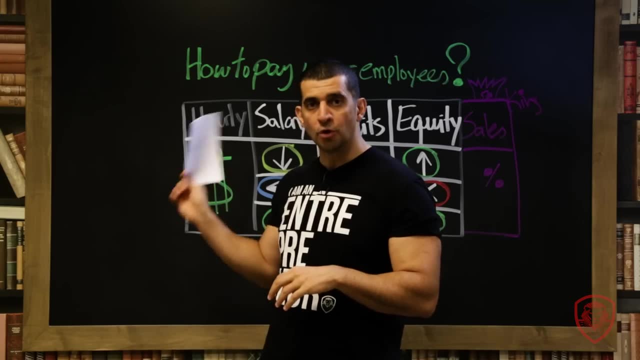 couple thousand salespeople that are working for you and executives. It's something you want to definitely pay very close attention to, So let's get right into it. In this video, I'll cover with you different ways you get paid to your employees and then 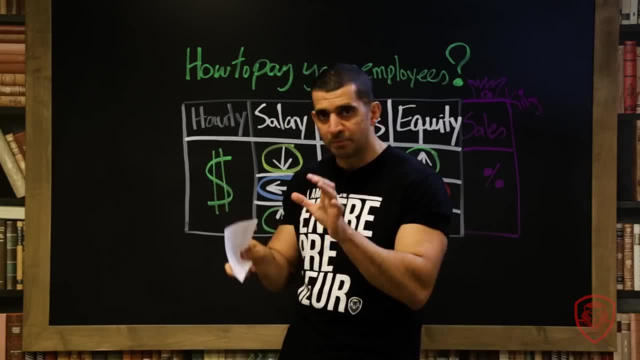 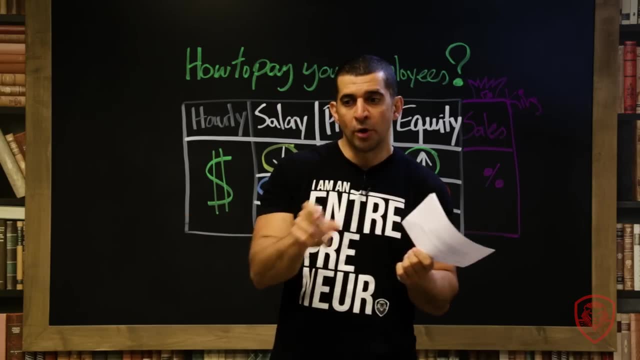 I'll also talk to you some strategies on what you could do and what's the best to combine with what I get asked all the time: How do I offer equity? Do I give this person salary? Do I give this person hourly? When do I pay them this? 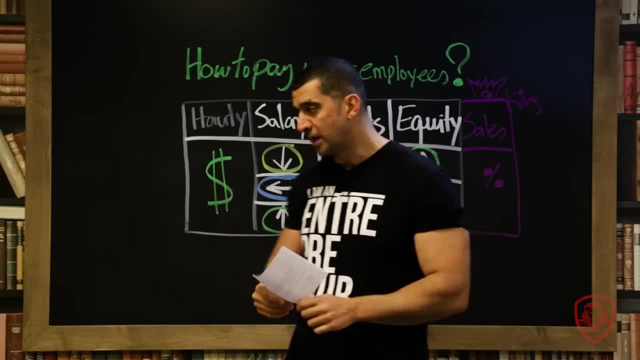 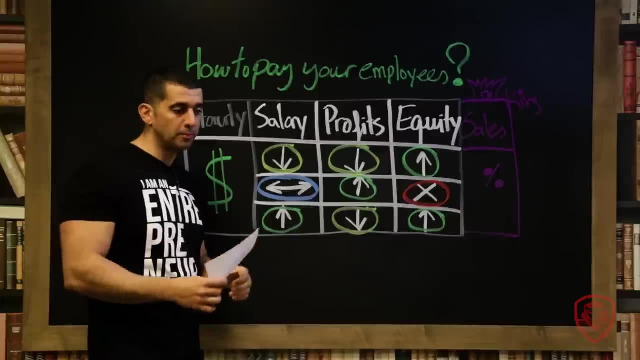 I want to bring this guy on board. Do I bring him on board now? We'll cover all that stuff together with you in this video. Okay, so let's start off. Simplest way is hourly employees. Now, who are hourly employees? 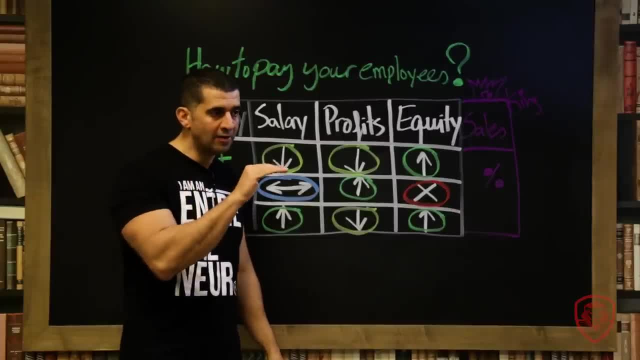 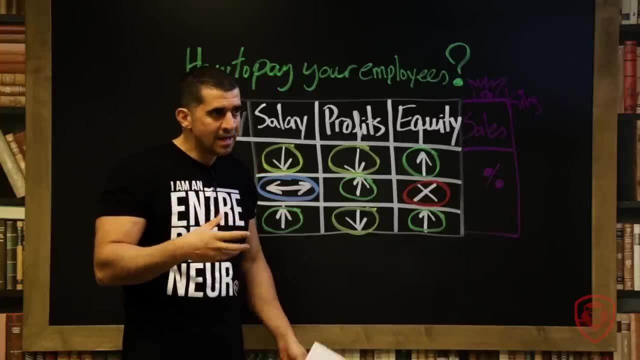 Hourly employees are typically people who have a very simple, low skill level job to do. For instance, when I worked at Haagen-Dazs, I had to learn how to make banana splits right, Or a sundae. That is an hourly job. 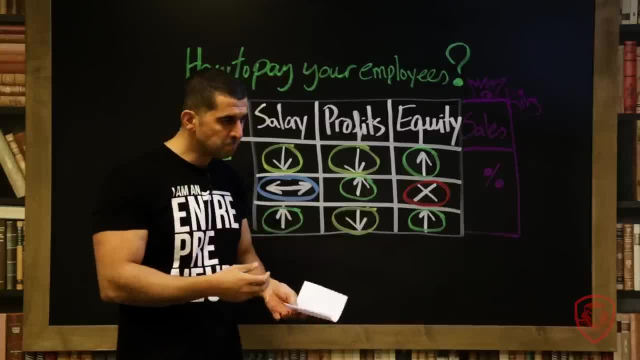 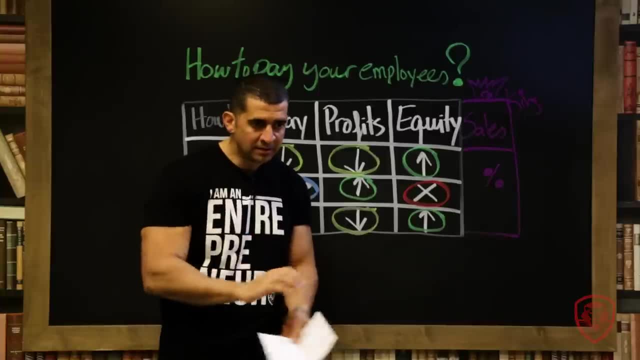 You're making $3.25 an hour is what I was getting paid, right? If I'm working at Burger King and I'm making a Whopper no onion, okay great. a Whopper no onion, Two buns, boom. This is a very easy skill set, right. 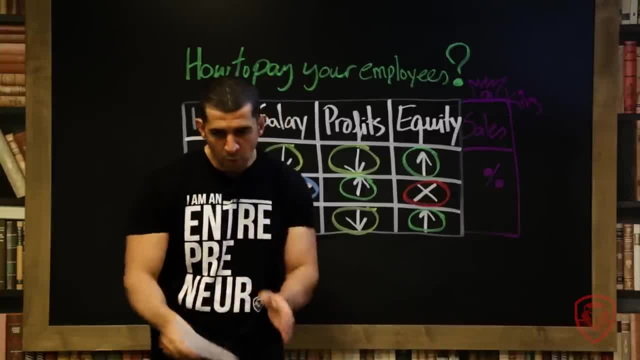 This is all I'm doing. That's an hourly $4.25.. If I'm working at Bob's Big Boy and I'm the busboy, all I'm doing is taking all the stuff and I'm bringing them. These are all the jobs that I had right. 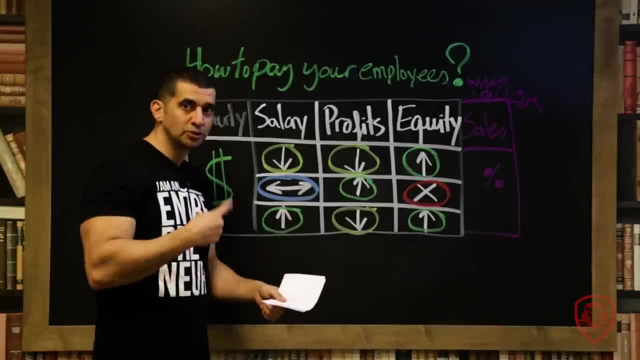 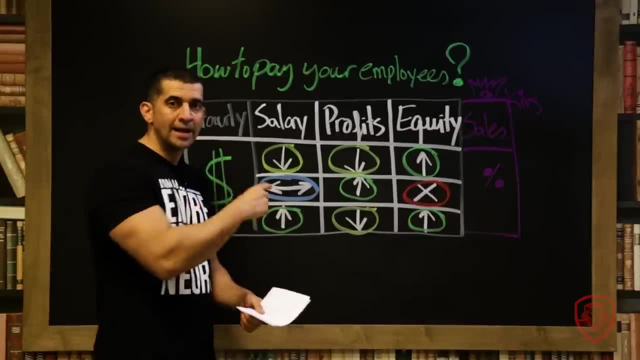 This is an hourly right, So it's low skill and it's just transactional- Low skill, transactional- And it's a very great platform for you to identify, For you to identify people that want to make transitions to the next level. 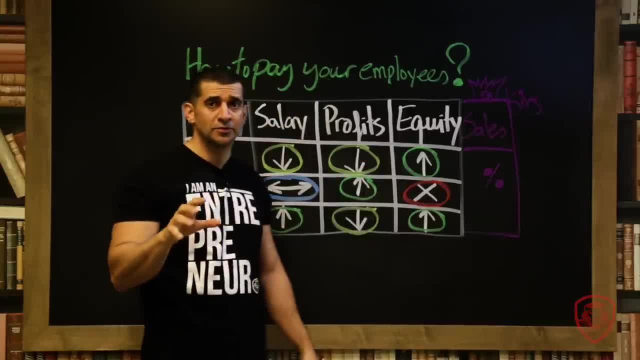 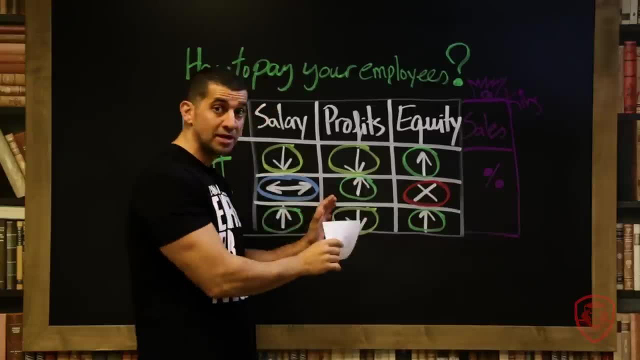 It's a very, very good filtering system here. And, by the way, whatever I tell you in this video, it's very important for you to abide by your state laws or your country laws, wherever you're from. So I'm just telling you simply stuff that I've done, but you've got to make sure you're. 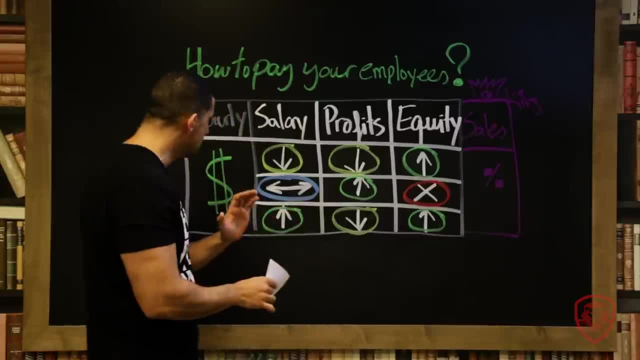 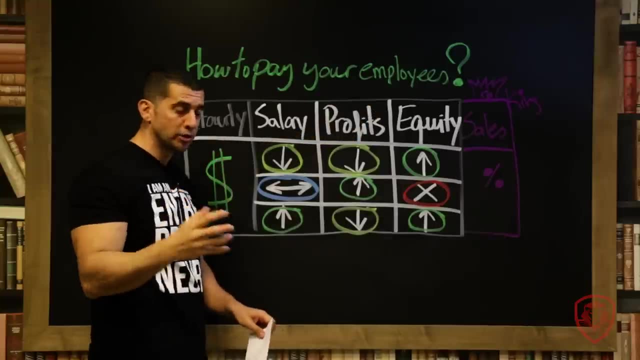 paying very close attention to your state human resource laws that you've got to follow. So, going back to it- filtering system from here where people go to the next level, It's also a great opportunity to see who the hardest working people here are at the hourly. 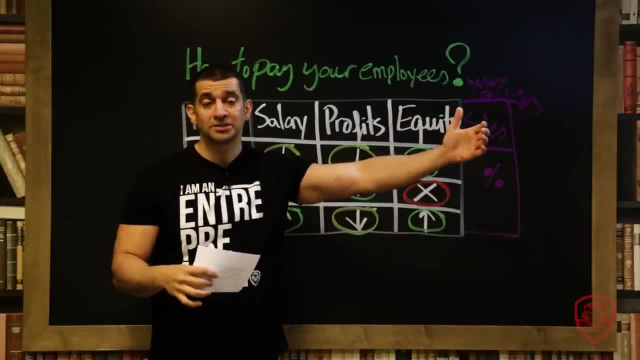 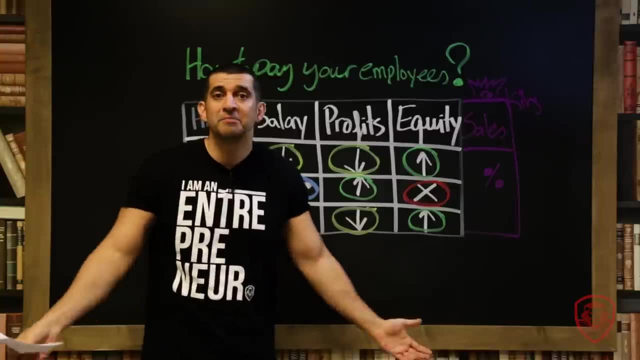 Next level Front desk clerk. You know we've had somebody who got started as a front desk clerk and then all of a sudden she was so amazing that she's been with me for 11 years now And she started making $800 a month initially, or $400 a month. she was working two days. 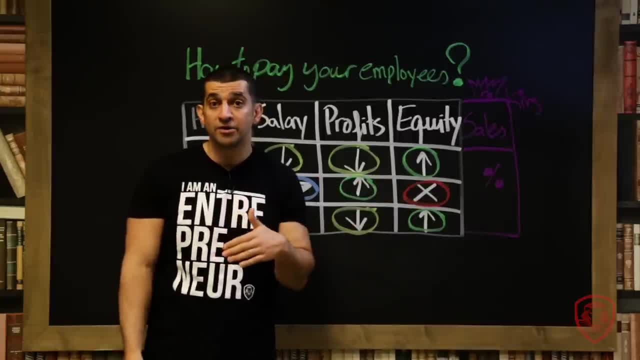 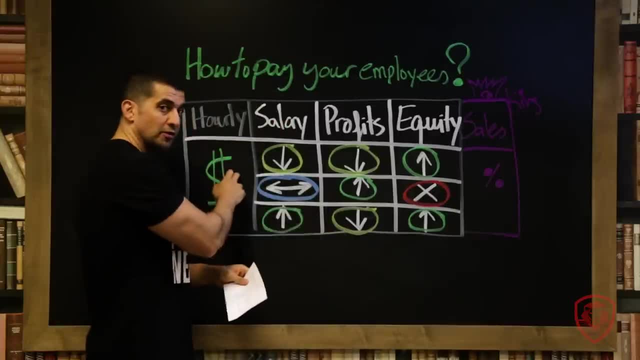 a week And the next thing you know she's been with me. She moved her entire family and her husband here to Dallas from LA. Husband comes, two kids come, But she started off here right Hourly, Simple Salary. 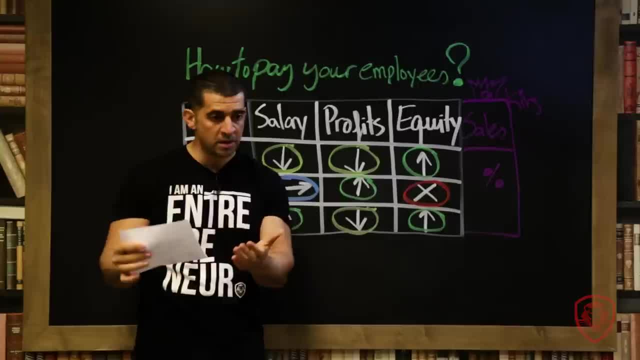 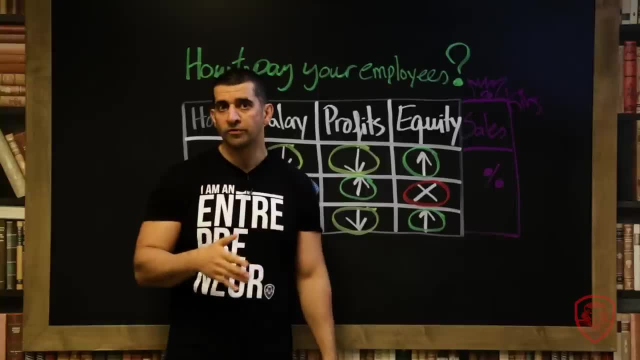 Salary is somebody that's more than hourly. It's somebody that you're telling them we want you to get a promotion. You are now a salary position person here in the company And sometimes salary is going to work more than 40 hours a week. 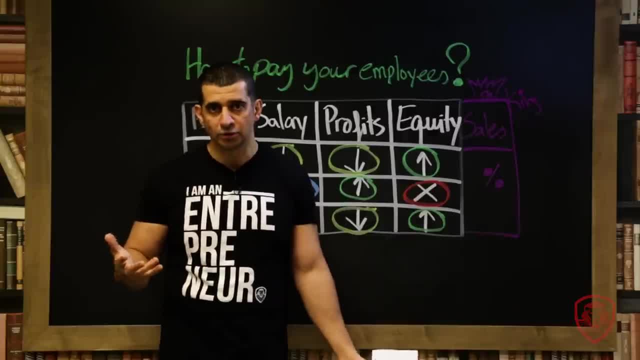 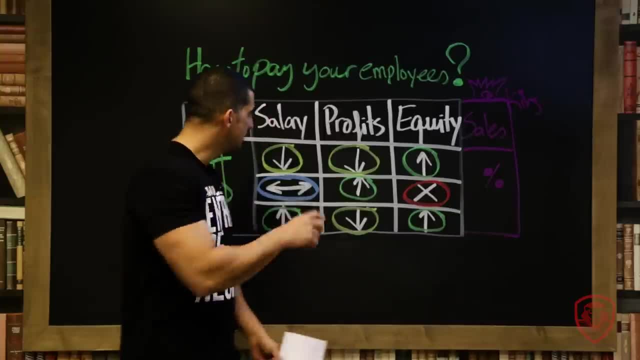 If I have a job that I'm working salary, you would never catch me working 40 hours a week. And here's why, If you're watching this and you're working only 40 hours a week as a salary, I like to go above and beyond, because I kind of want to get to the next level and the next level. 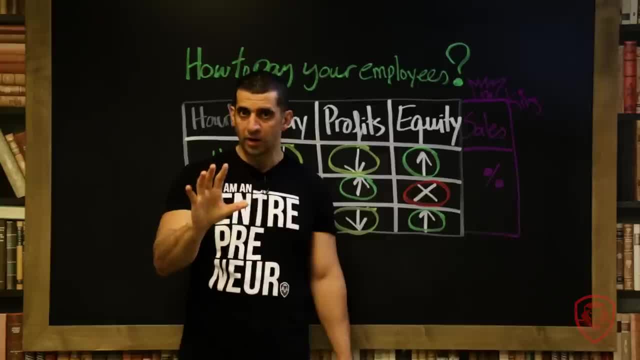 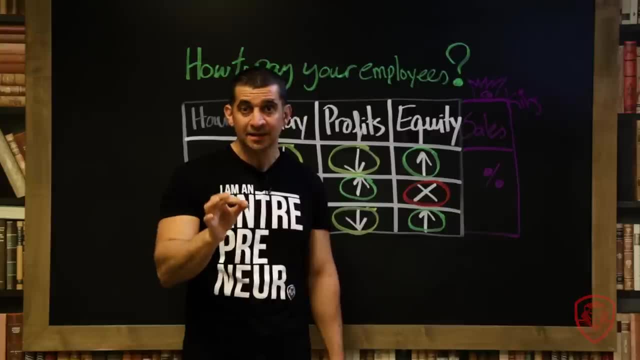 and the next level, And I want to have leverage when I'm negotiating my salary or whatever I'm doing. By the way, My own employees watch these videos. I teach my own employees how to ask raise from me. Every one of them who has asked for me in a raise, I've prepped them. 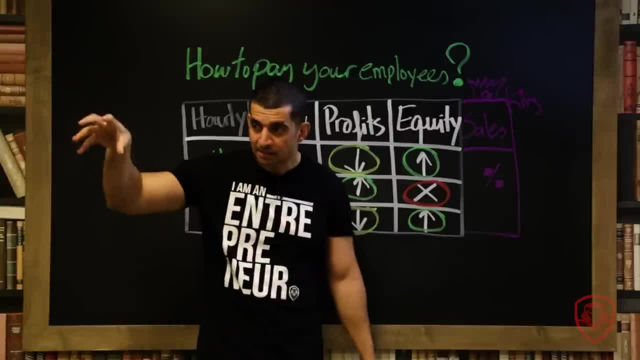 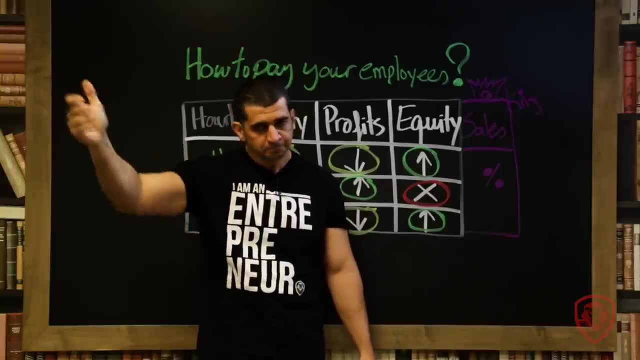 Here's how you ask for a raise from me: Dot, dot, dot, And they'll come and they'll present PowerPoint. Pat, I believe I deserve this. Tell me why. Pop, pop, pop. Nope, I disagree. Yes, I agree. 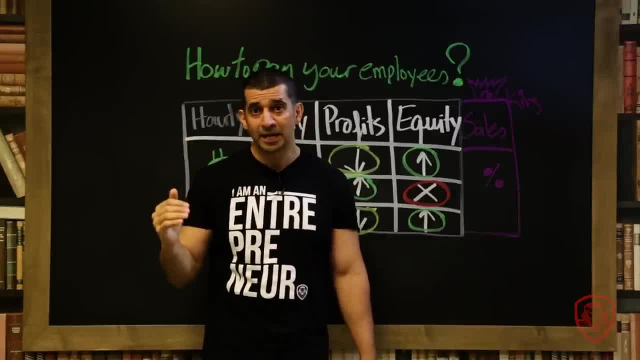 One time somebody said: I deserve this. I even gave more than they thought they deserved. And one time somebody asked me for something and I told them: no, They didn't get anything and I asked them to leave. So it's both ways, But it's transparency. 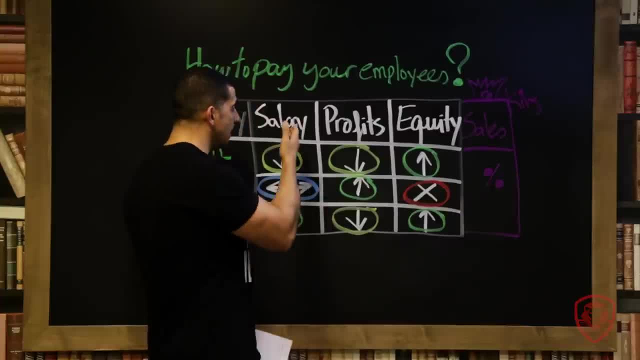 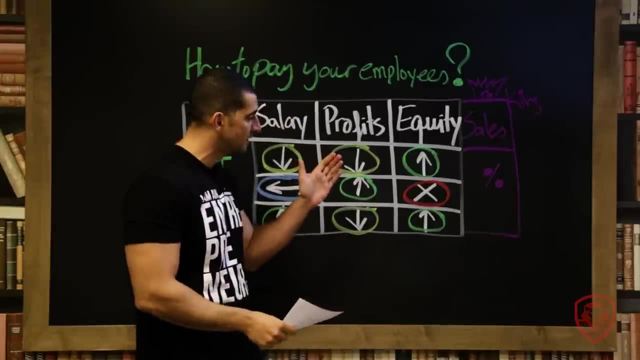 So salary is the next level. Then you have profits. What's profits? Somebody who's getting paid salary plus profits. Why is this important to give somebody salary plus profits? Because salary plus profits allow somebody to scale Like they are willing to work a little harder and push a little harder on a Saturday. 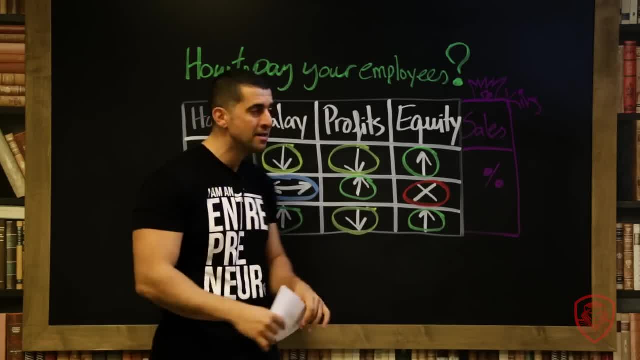 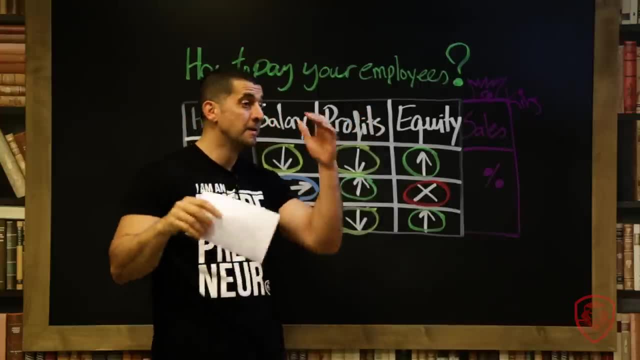 Or the effort is paying attention to more of the details and they're rallying everybody because there's a profit to participate in And this could be profit slash bonus, So you can change this profit to bonus. I'm participating in a, you know, tier level business. 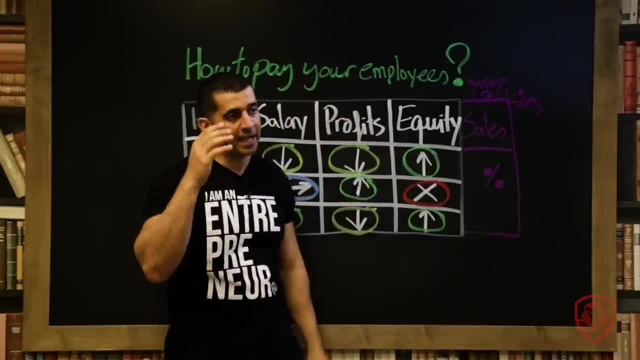 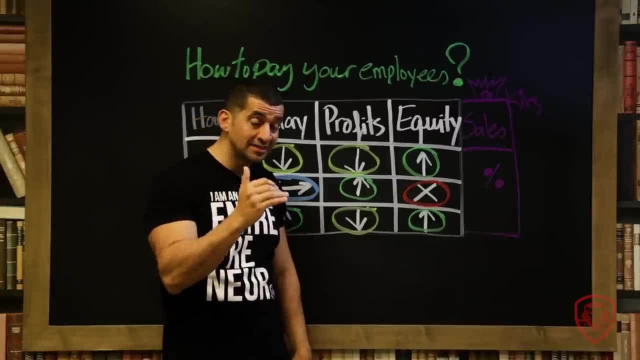 Level bonuses and profits. Let me explain here. If you hit XYZ, you're going to get a $5,000 bonus. If you hit ABC, you're going to get a $10,000 bonus. But if you hit this, we're giving you a $25,000 bonus by the end of the year. 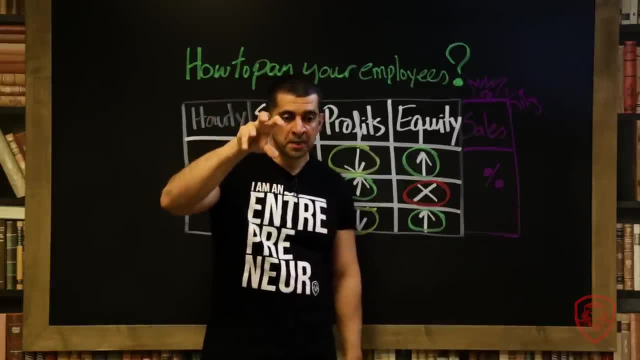 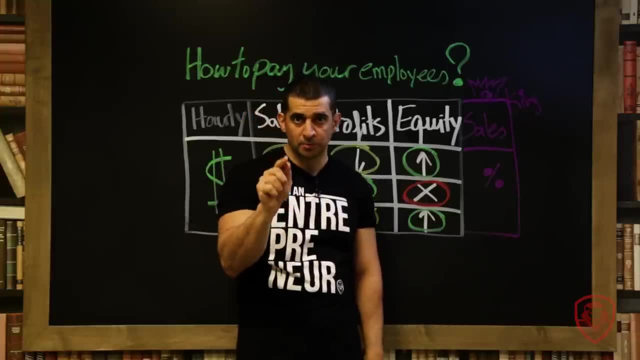 And then it comes down to how you put the ABC bonus together, where it could be that you're going to get judged on how well you create the bonuses, Because the bonuses comes down to you, how creative you can be in that area to get them. 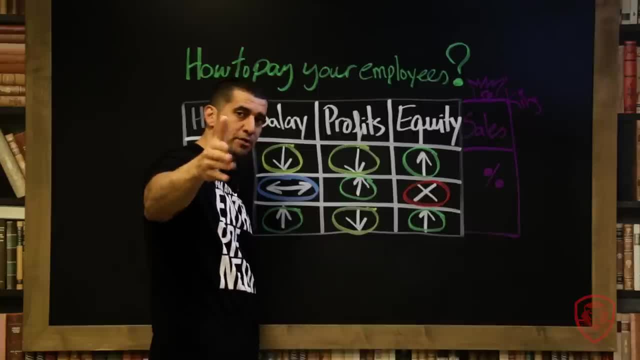 to pay attention to areas that matter. What is the most? increase the value of the company, if that's what you're looking for. Increase the revenues of the company, if that's what you're looking for. Increase the subscribership of your company. 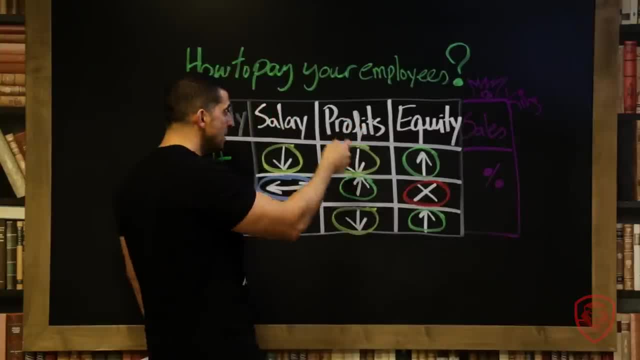 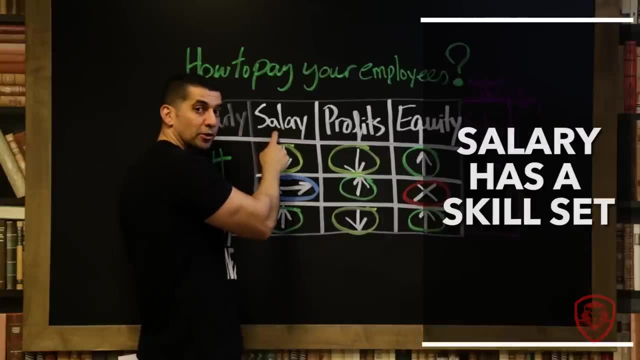 Whatever you're looking for, This is a very important thing to put. Now, if I go back to the salary, the difference between hourly and salary: A salary has a skill set. Hourly doesn't necessarily There's a skill here. 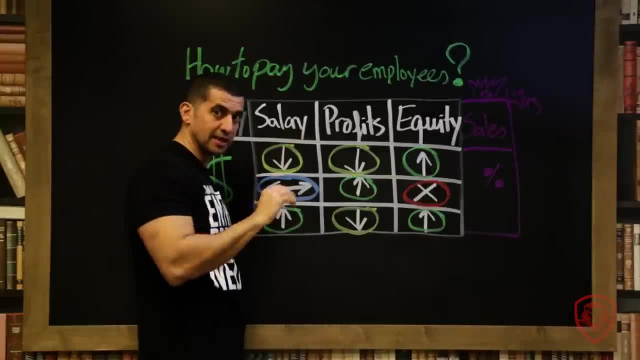 There's actually a measurable skill set that this person is bringing to the table, And then you have equity. When do you give equity? Equity is a matter of choice, And so when you give equity, equity actually is based on your current income. 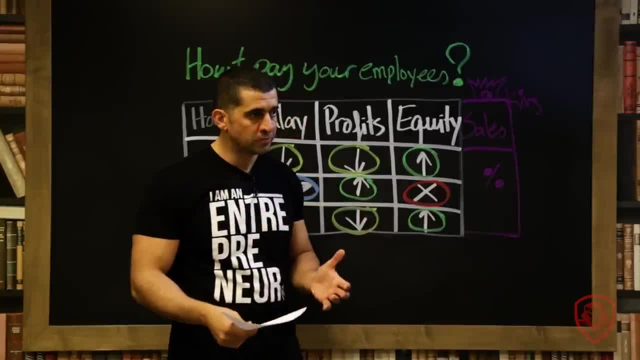 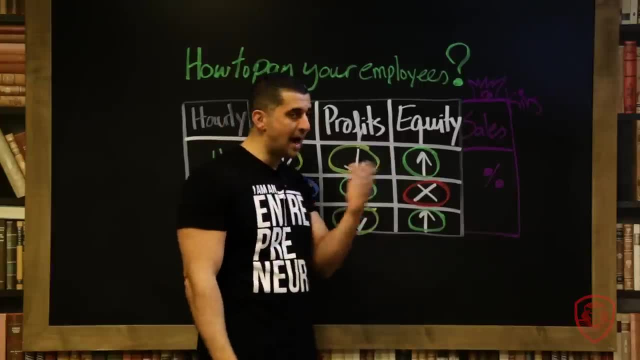 When you give equity. equity is based on your current revenue base is, eventually, if you want your best executives to come on board and work with you, and I'm a fan of equity. Some CEOs don't like equity. Some CEOs prefer to get profits. 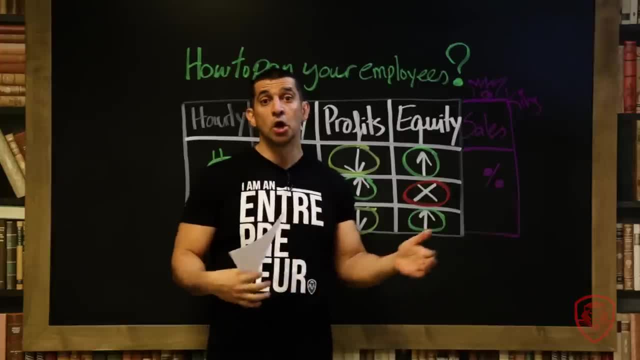 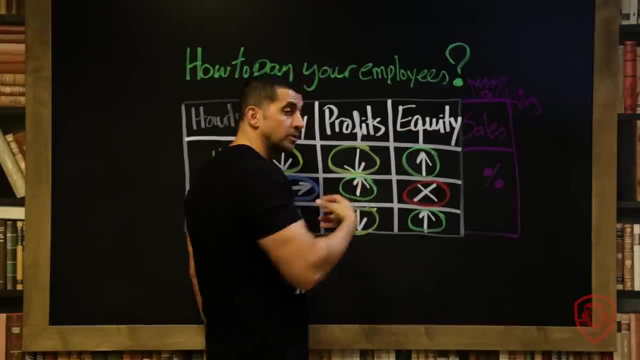 Some employees don't even want equity because equity to them is long term. I like equity because equity gets me to know if this person's a long term person or a short term person. If I offer equity or a person's asking me, Pat, I want a piece of the company. don't. 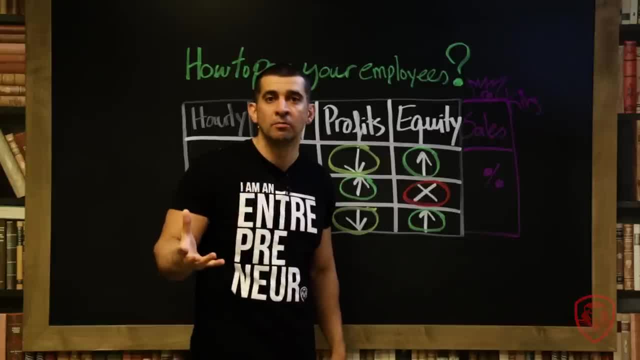 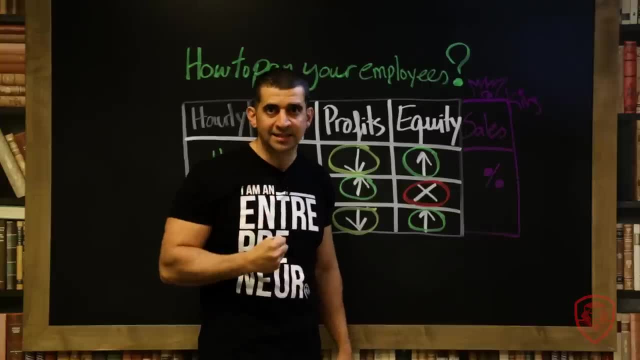 get offended by that. That's a compliment. Hey, I want to be with you long term. It's like a girl saying: when are you going to put a ring on my finger? That's what equity means. If someone says it to you, take it as a compliment. 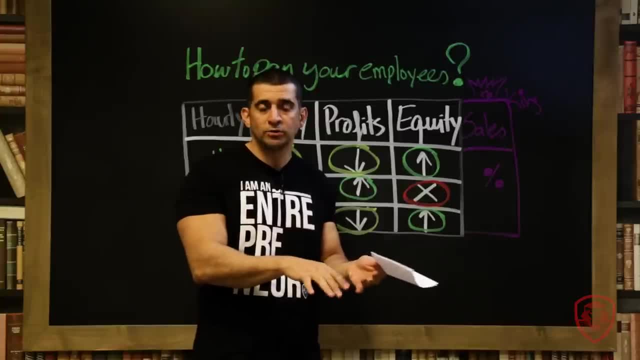 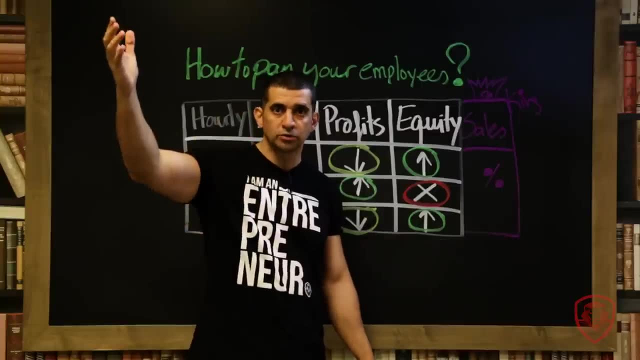 Don't get upset and message me two o'clock in the morning saying, Pat, what do I do? This person's asking for equity. I think he's going to leave me. They're not going to leave you, They're simply just asking you: what can I do to participate in the bigger victory? long? 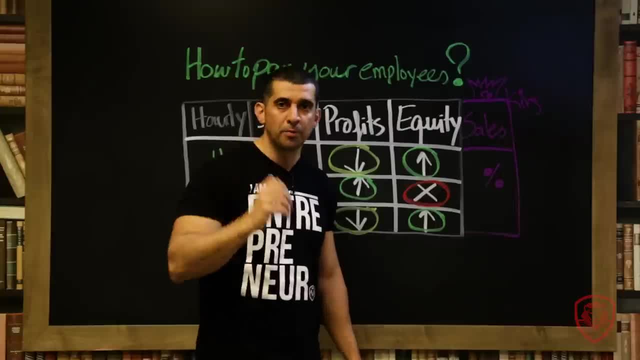 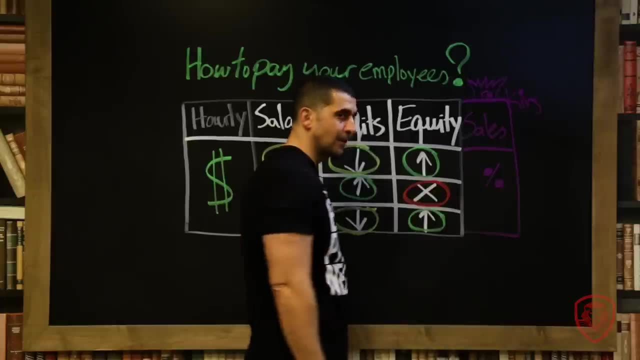 term with this company, Because I love this company. I want to participate long term, No problem. So that's the equity part right, And you'll determine who to give that to. I'll explain to you here in a minute, And then it's sales. 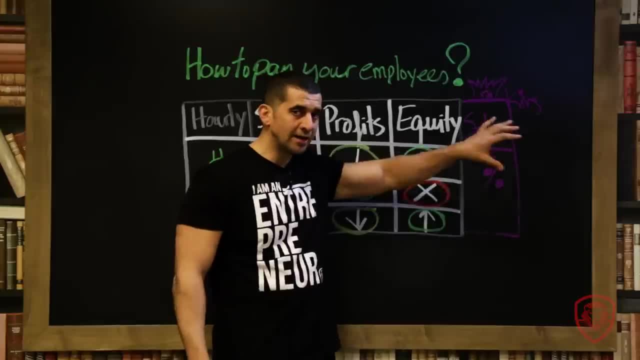 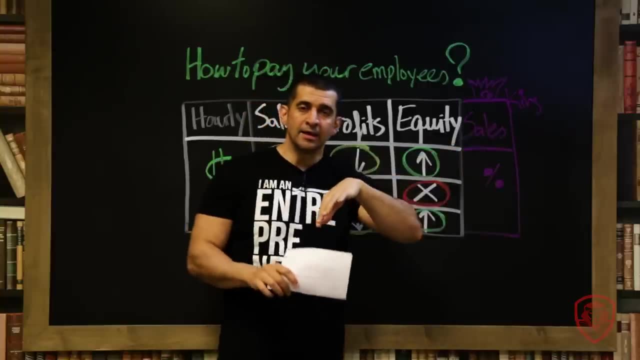 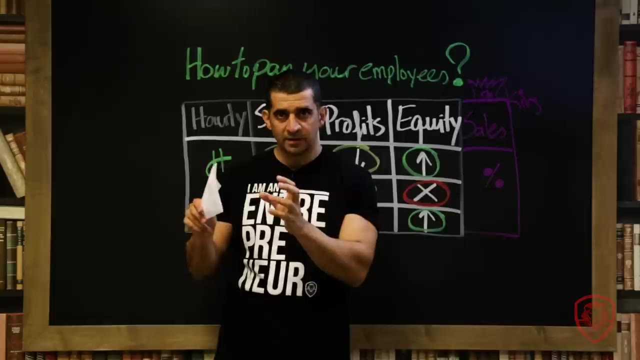 Sales is very simple. Sales is king. Without sales, nothing exists. Without sales, nothing exists. I put the crown up here. these guys run the entire show. Google without pay per click does not exist. Okay. Facebook without the advertising and the boosting doesn't exist. 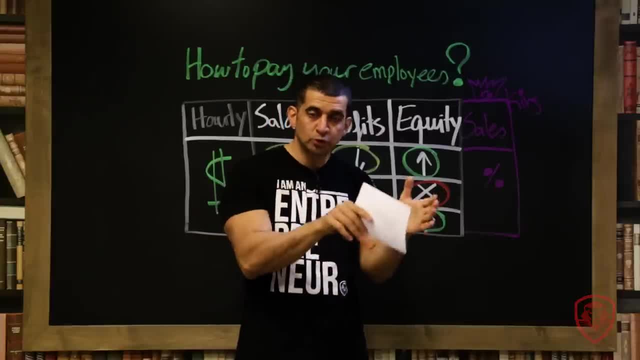 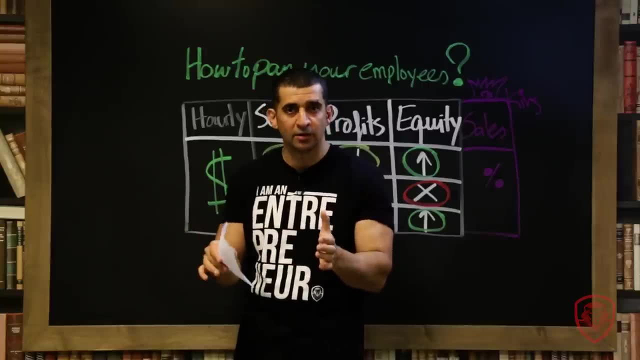 Doesn't exist, That's sales. Sheryl Sandberg brought sales to Facebook. Okay, If there is no sales, Keller Williams doesn't exist without their sales people. Gary Keller has built an incredible organization with nearly- I want to say it's- the 90,000. 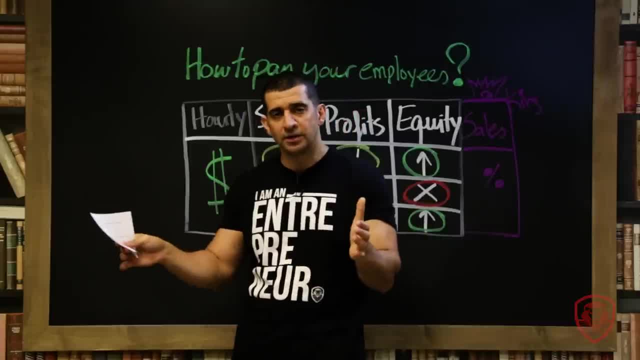 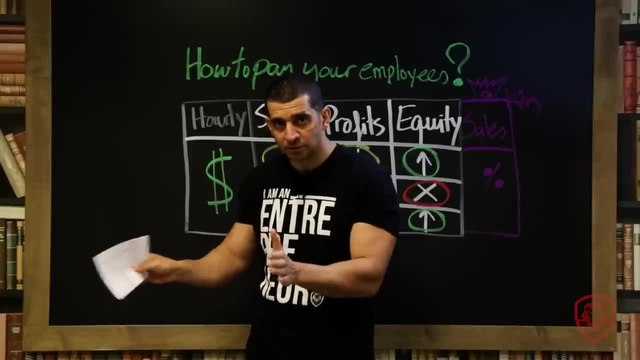 real estate. they're the largest real estate brokerage house in America And he wrote this book called The One Thing Phenomenal Book. There is nothing with Keller Williams if there isn't sales, Nothing. Sales is king In every company. sales is king. 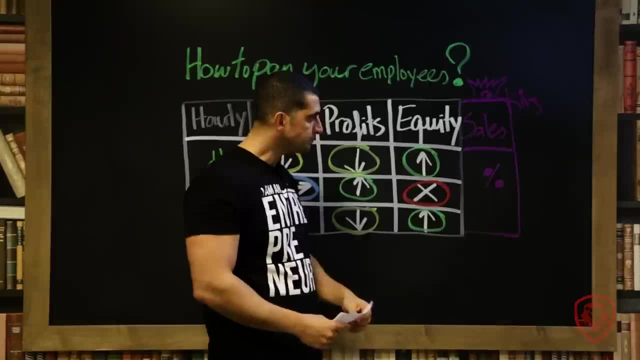 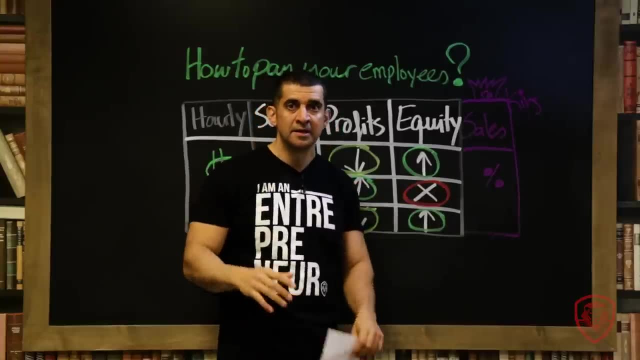 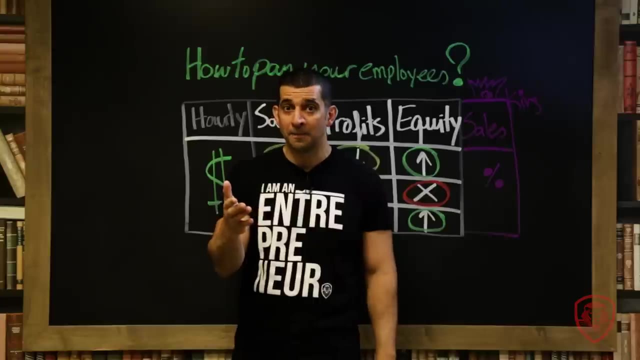 So your commission structure in sales needs to be set up in a way that you're going to be judged on how you set up your commission structure with your company, because if you don't do it right, then you could potentially incentivize bad habits. That's on your comp plan. 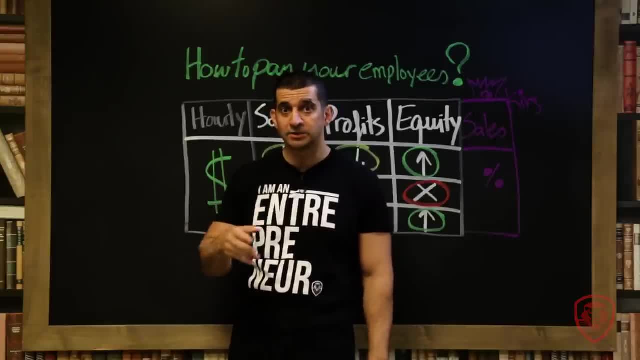 We've made this mistake before myself in the past. This is why now a lot of people call and say, Pat, can I come with you and meet with you and have you help us put a structure or a comp plan? I don't have time to do it. 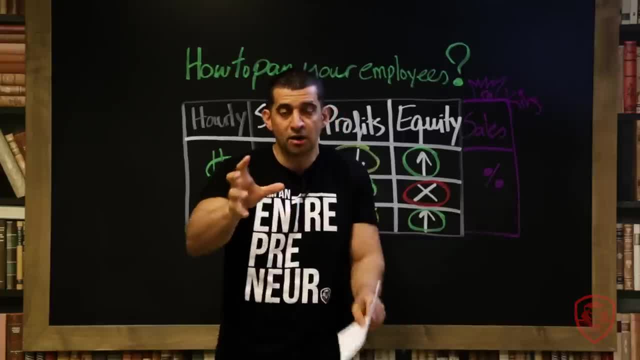 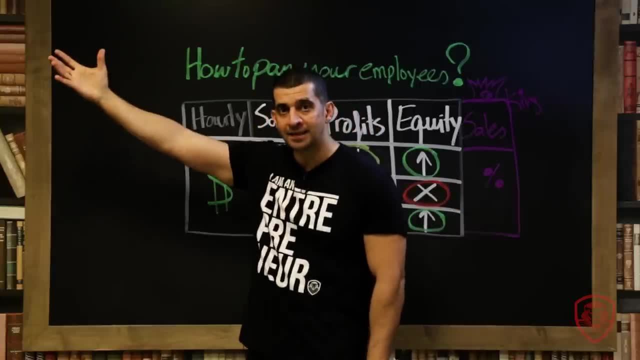 But please help us. I don't have time to do it, But just go back to yourself and think about the way you set up your company. That's the key. Your comp plan: what behavior do you want me to get? that again goes back to increasing. 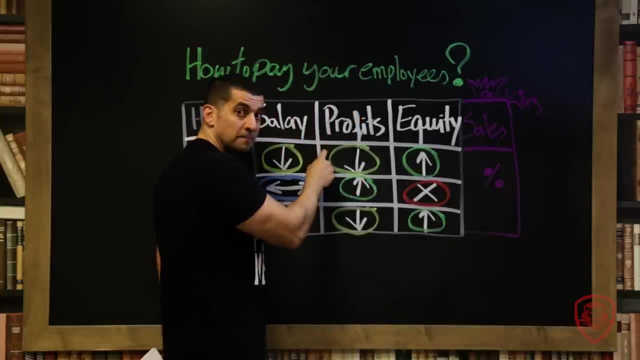 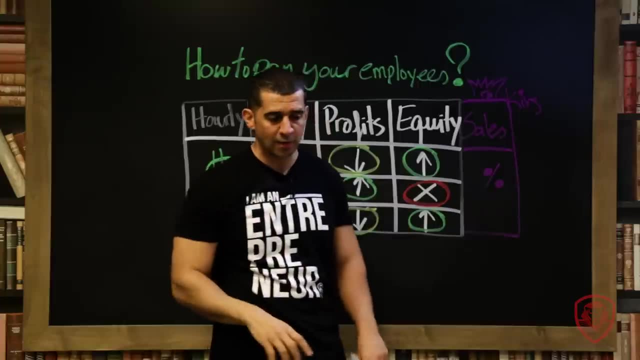 the value of what The company? Remember how I talked about bonuses here, or the profits. Remember how I said: what behavior do you want from your salary employee to get them to do above and beyond? Same exact thing here? What behavior do you want for salary, for commissions, for them to do very well? 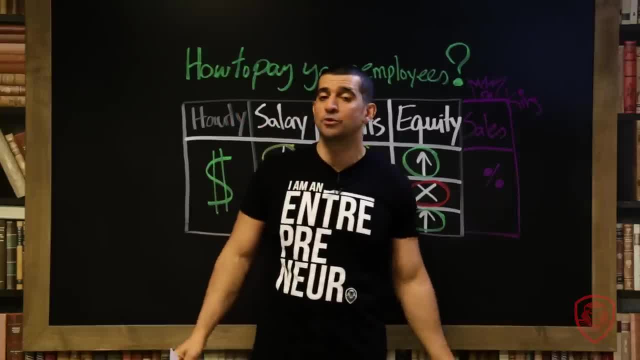 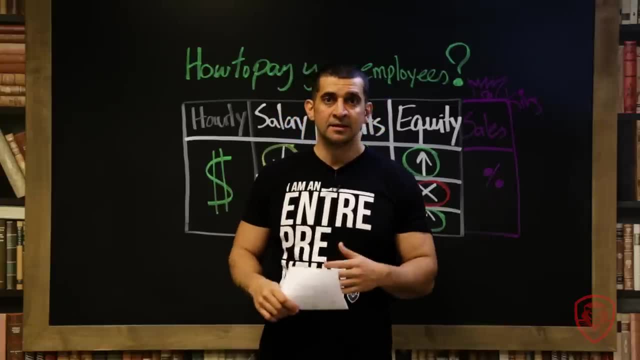 And then their comp plan. when it comes down to sales, I don't like caps on how much money I can make. Some companies put caps. I'm not a fan of caps. I sit on a few. I sit on a few boards and some of these guys want to put. I don't think this person needs. to make more than $400,000 a year. What if they make more than $400,000 a year? What if a salesperson makes $1,000 million per year? What if a salesperson makes $2 million per year? That's totally fine. 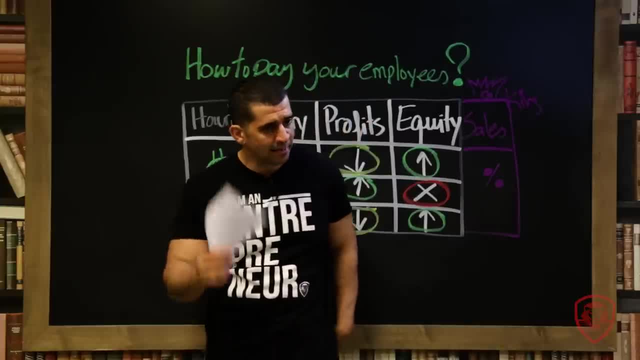 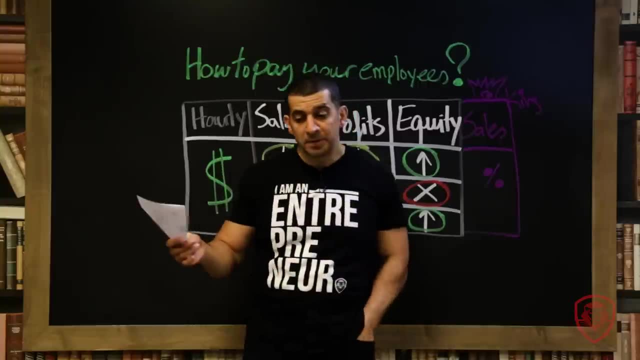 Don't put a cap on sales. My suggestion don't put a cap on sales- And I know the logic behind some people who say I want to put a cap on commission sales- is because I don't think if these guys make too much money they're going to lose. If they make too much money, they're going to leave me and be a competitor of mine. Sometimes, if they don't make enough money, they may leave you and go be a competitor of yours. So what if that happens? I don't want to put a limit on this side. 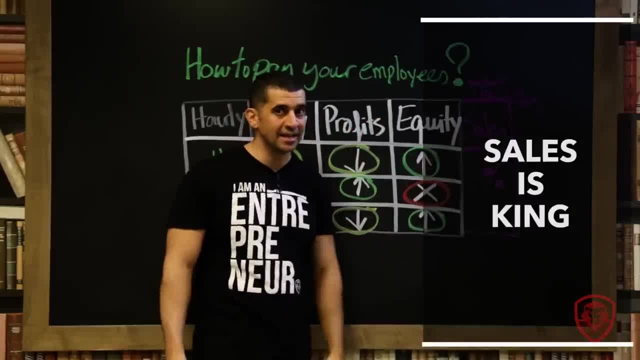 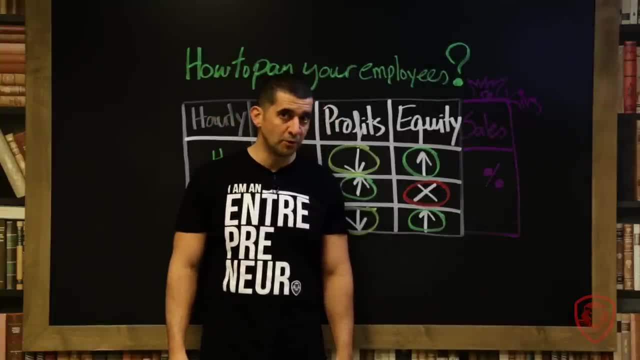 So sales is king. The tough thing with sales is king is I had a company that brought me in and I spent a full day with them and it was very, very painful to be around them, because they're asking: how can we grow the company, and this is a multi-billion dollar company- how can we grow the company? 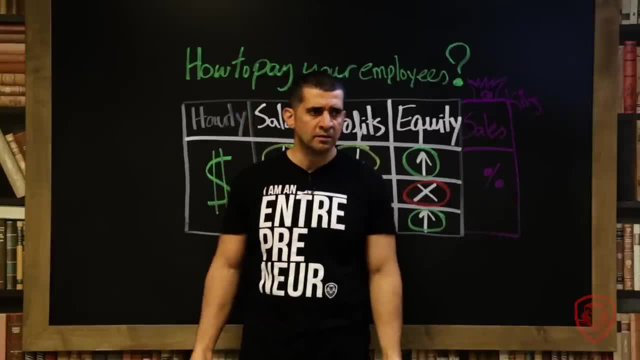 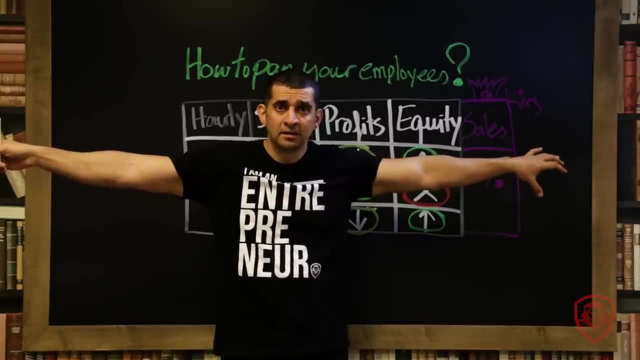 oh, we don't want to change our comp plan, but tell us how can we grow the company? I said first of all, your comp plan is set up in a way to only favor the sales people that have been here for 25 years and they're not working. 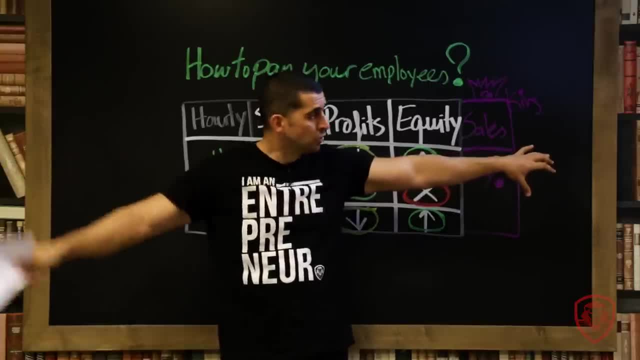 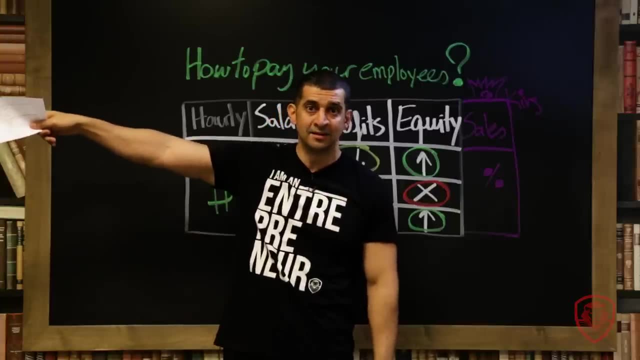 They're not getting off their asses. You're not moving this company. Your entire incentive plan is to get those guys to just manage Your best. sales people are not selling. That is a terrible compensation plan for your sales people. But no, if we do this, they're going to leave us to another company. 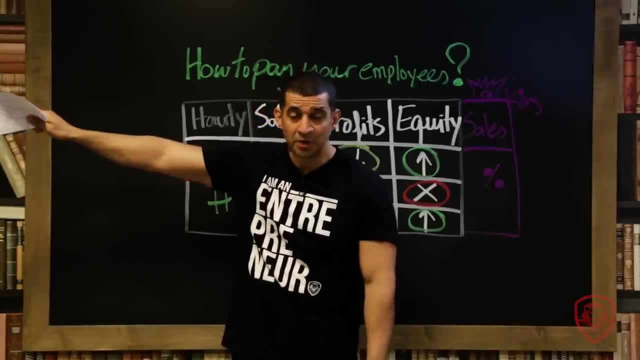 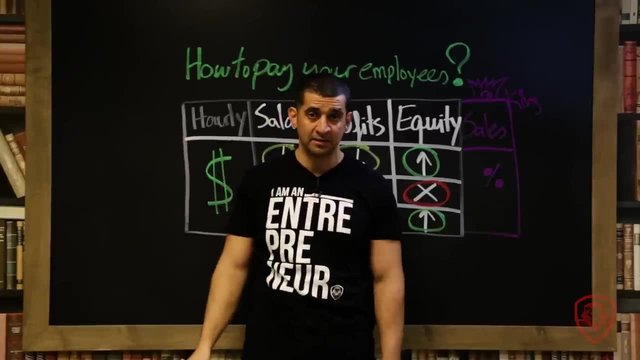 Let them leave. They're not going to leave. They're afraid of working. They haven't worked a 60 hour work week in 10, 15 years because your comp plan makes them lazy, Comp plan produces lazy people And comp plan produces leaders. 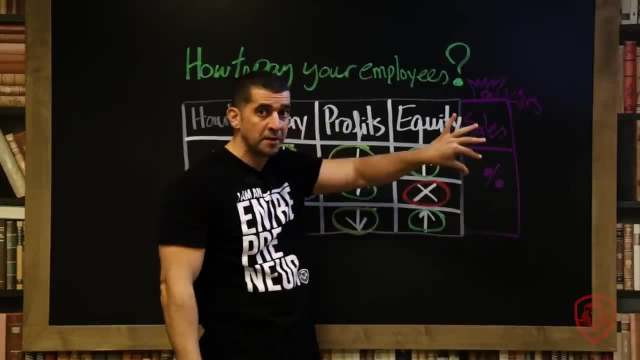 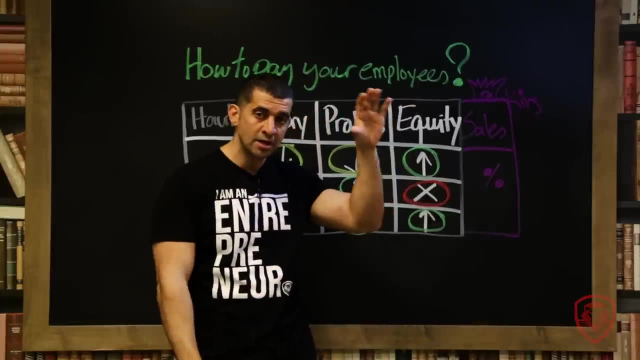 Comp plan produces managers and comp plan produces leaders. So it's very, very important There's an art to how you set up your comp plan properly, where they're not breaking the rules but they're growing your business. So we may come back to that here in a minute. 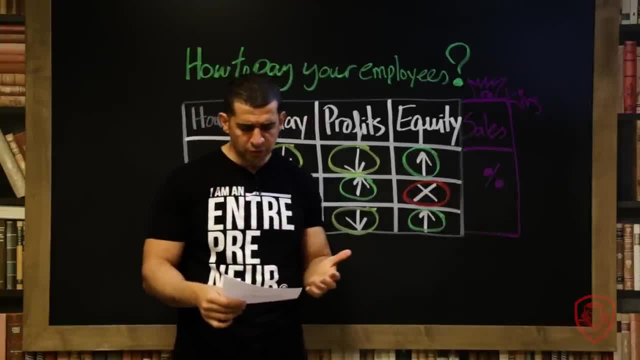 And talk about it. So now let's talk about it. You may say, Pat, so what do I do when I'm hiring somebody? and I kind of want to be able to know. this person is saying: do I do salary plus equity? 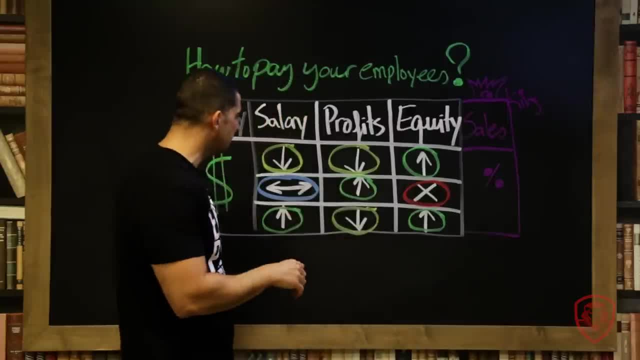 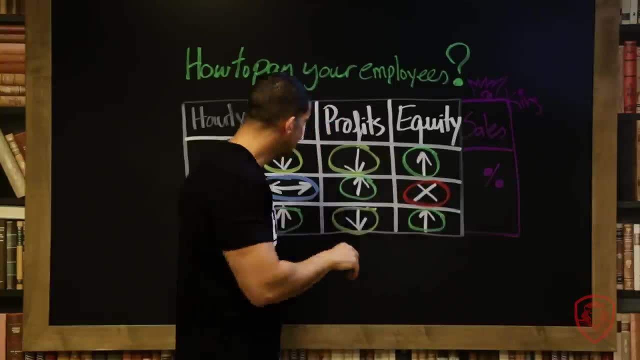 Do I do this plus that? What do I do in this area? Let me kind of give you an idea. If somebody says, Pat, I want equity, No problem. I've had negotiations with many of my employees: Pat, I want equity. 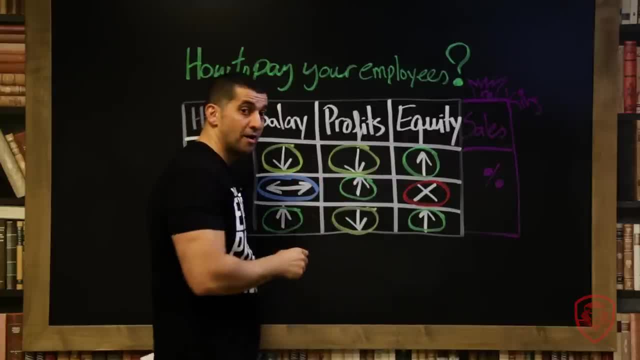 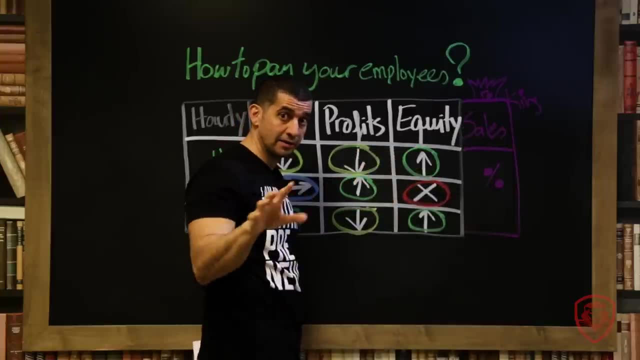 Great. So I want equity, I want salary and I want profits. It doesn't work that way. If you want equity, Let's talk about it. If you want equity, long term, victory. great, I like that. Welcome. Your salary's probably going to be low and you're probably not going to participate in. 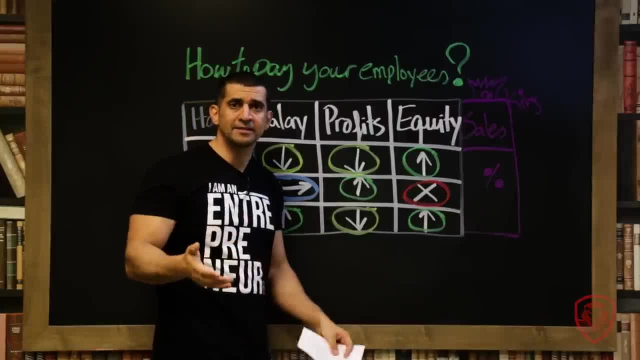 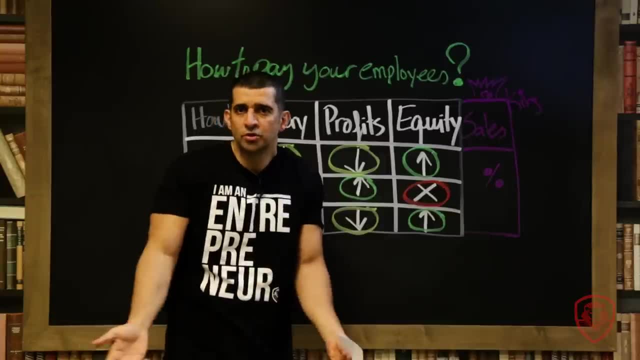 profits, Initial stages, Obviously, at the end of the day, when the company starts profiting millions on top of millions on top of millions of dollars, it's a mathematical formula. You're going to participate in profits if your department's doing their part. 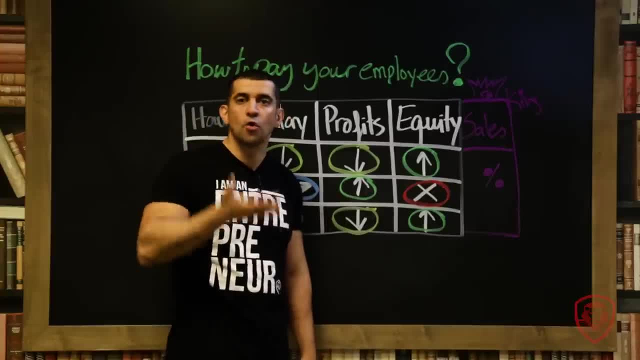 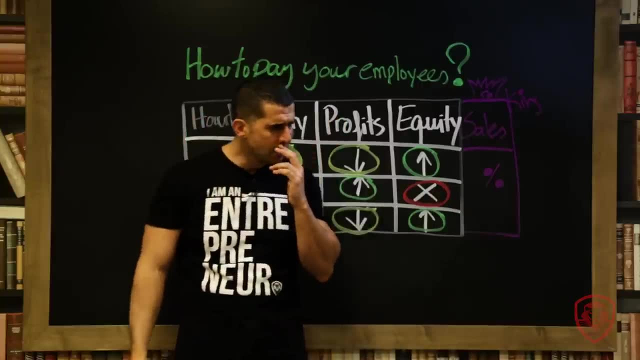 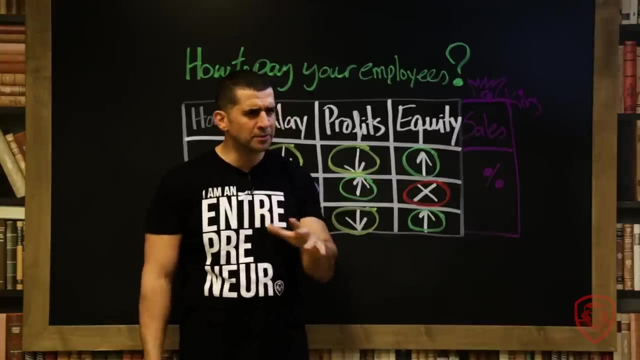 Great thing about capitalism: it's all math. It's all math. Money flows, Money flows through and everybody participates. If you can prove, I'm having meetings with a different department of ours- I think every single department had grown by 130%. every one of them had grown by 130%. 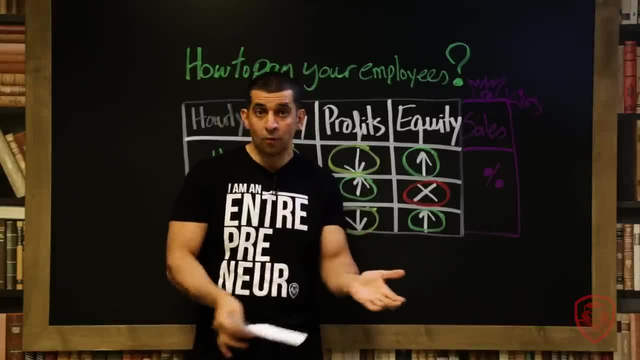 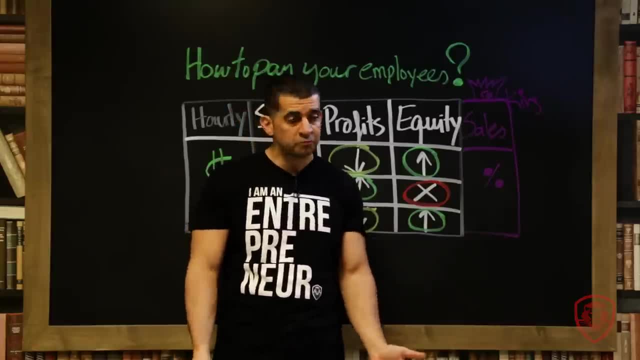 or more give or take, except for one. And I told that one person we were talking. I said: you don't have no leverage. Your department is a department that has not grown. It's a measurable number And you know he came back. you're right, I've got to work on it. 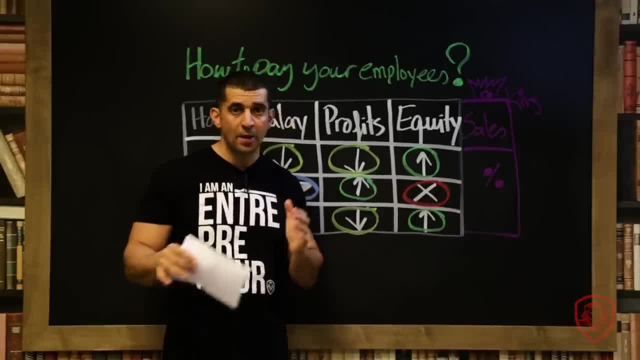 Great, He's going to go back and work on it. The feedback was given on being proactive and, instead of being reactive, you're just waiting for us to tell you what to do, and you're no longer being proactive. You used to be and you're taking a hit. 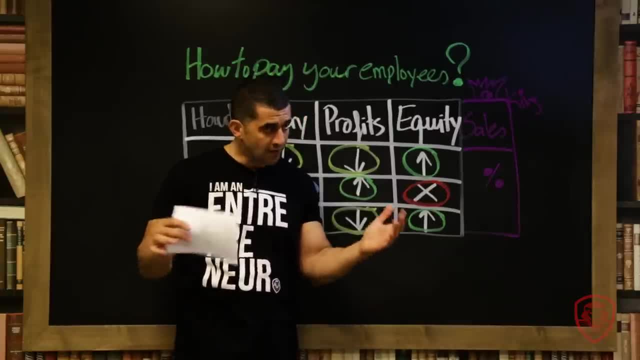 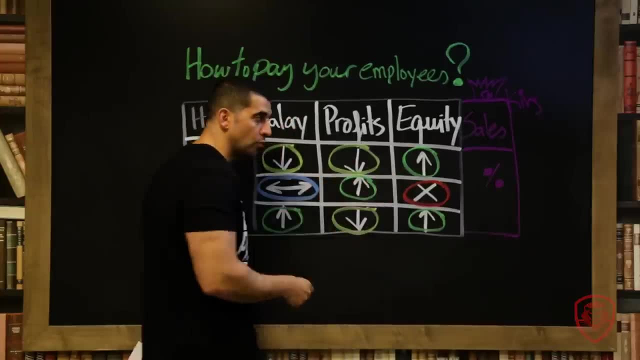 And, quite frankly, this behavior cannot continue. You're affecting the entire team, Fair enough. So you've got to have that conversation. It's not just a one-way highway, Both-way highway. So if you want low salary, you want low profits, we'll give you equity. If you want equity, you're going to have this. Or somebody says: well, I want a decent salary, but I don't care about equity, I want to participate in bonuses this year. Okay. So instead of getting a $40,000 salary, you want a $50,000 a year salary. 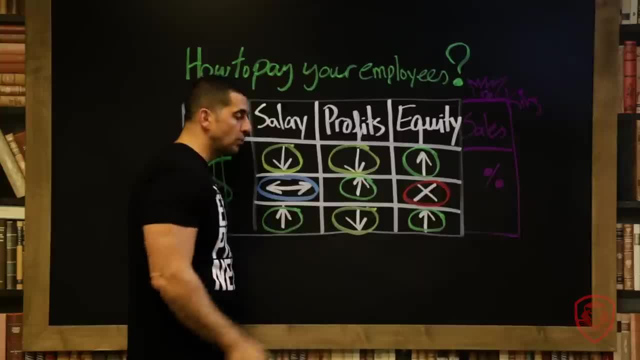 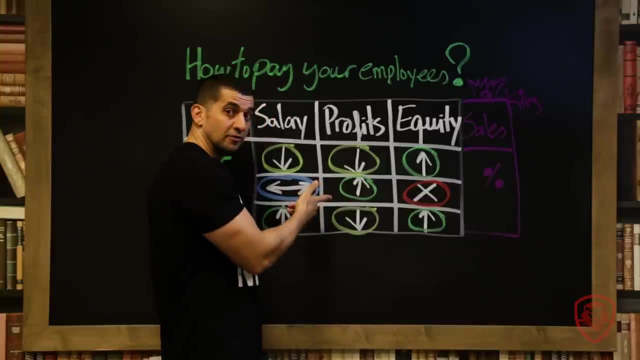 But you don't care about equity. I want to participate in bonuses this year. Okay. So you want to be able to bonus $20,000 this year? No problem, We can work that out. But zero equity- Great. Which means at any point this person can leave and go elsewhere. 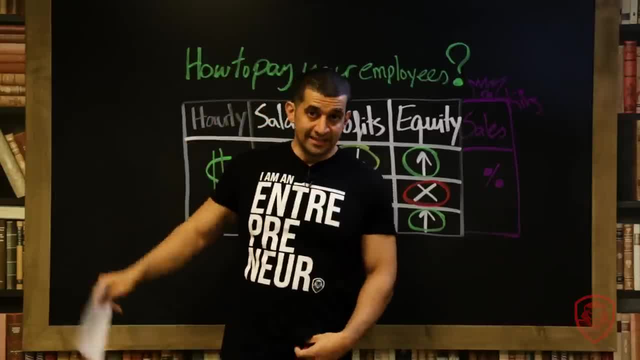 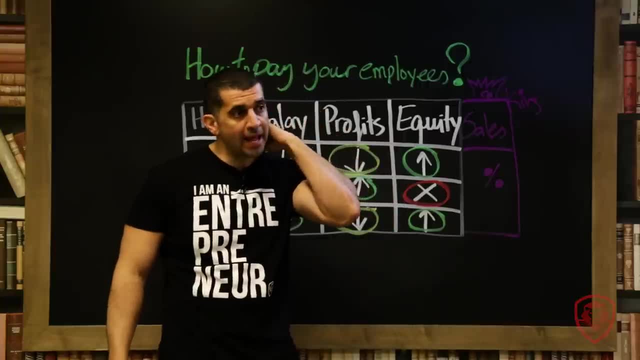 Or this person may have some issues: tax liens, they may have unpaid child support payments that they want to pay off, or they have certain debt they owe to somebody that they just want to pay it off and they have to fix it now. 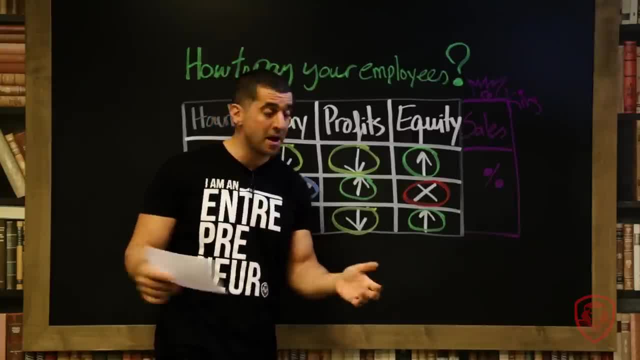 And you don't know the whole story. They don't want to open up and tell you about it. quite frankly, That's fine. They're motivated by the bonuses, right? So, red, there's no equity. They don't care for equity. 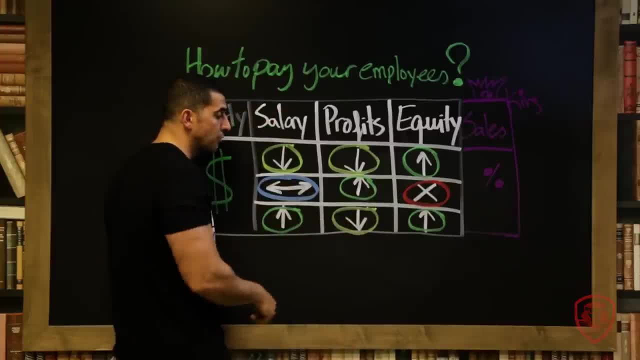 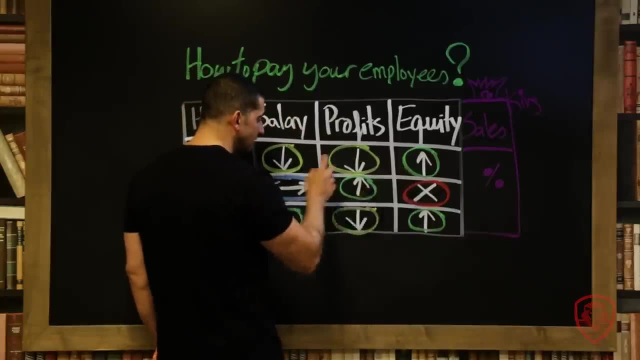 Great. This person may come and say: I want high salary, I don't care about bonuses, I want to participate in equity. So what's the difference between this and this guy? Because this guy wants equity, but he's getting low salary. 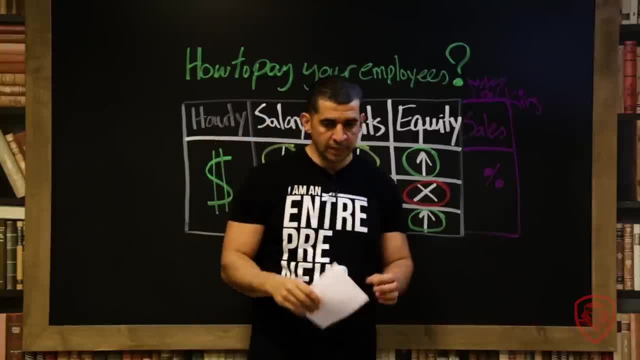 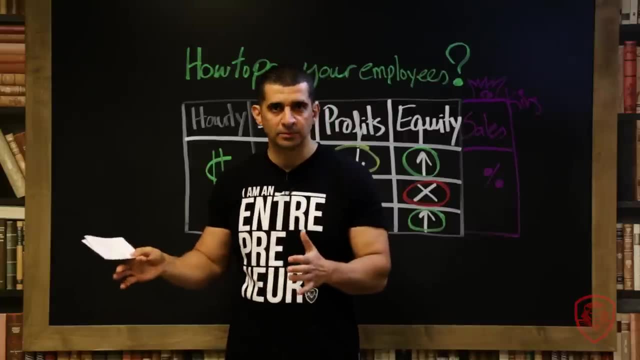 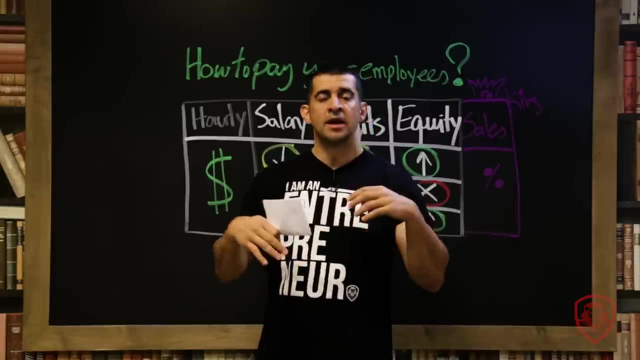 This is when it gets interesting. So in the world of sports, there are salary caps. let's just say, Right, There's always this collective bargaining agreement that they have in NFL and NBA and all this stuff and they come together. And any time you hear when there is a what do they call it a lockout? 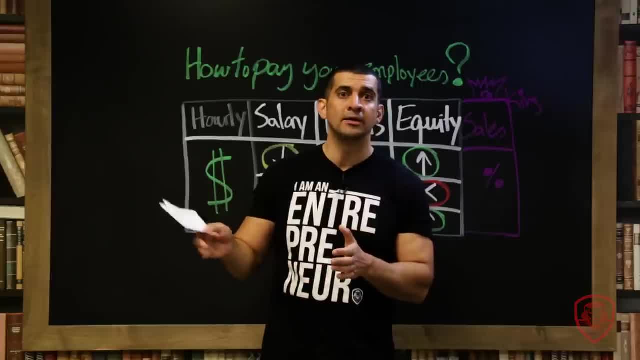 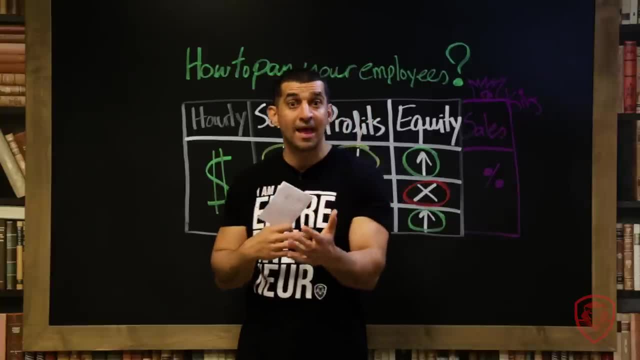 They call it a NBA. when no one's playing and they're renegotiating The collective bargaining agreement, there's a NBA lockout or something where they're not playing. Hey, they're not playing 30 games. okay, Because we're renegotiating. 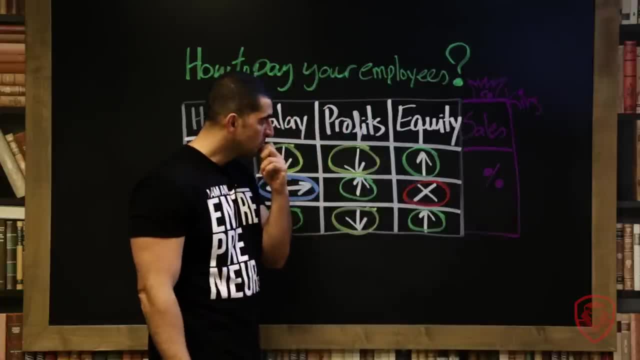 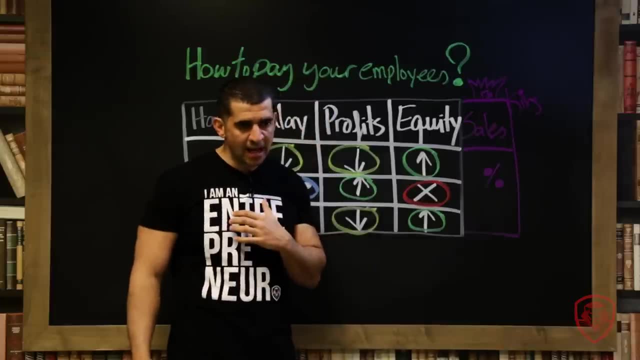 Strike, there's a strike, then there's a lockout. Yeah. So Sometimes, as an athlete sports team, you may be sitting there saying: well, wait a minute, I'm the Cavs. LeBron's contract is coming up with Miami, listen, let's pay him. 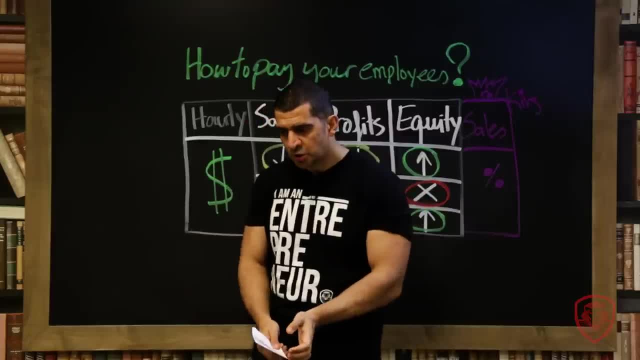 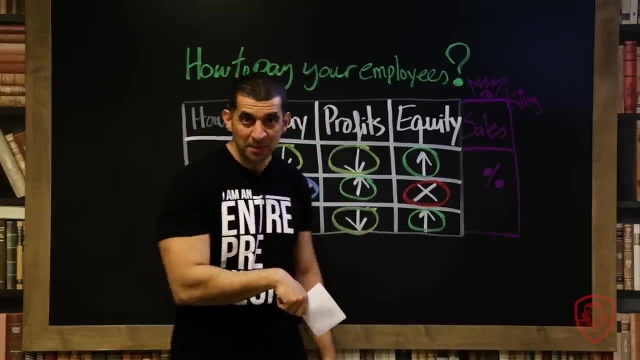 Who cares Right? Sometimes you're the Lakers', Jerry Buss, and you've got a Magic Johnson that's coming down from Michigan State and you know he's going to be a player, and Larry Bird is coming out, he's going straight to Boston from Indiana and you're bringing Magic Johnson, who's a 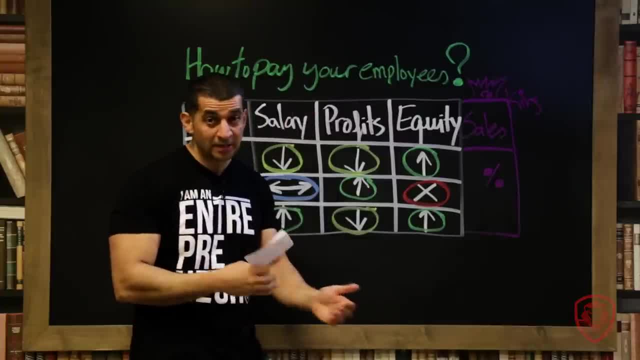 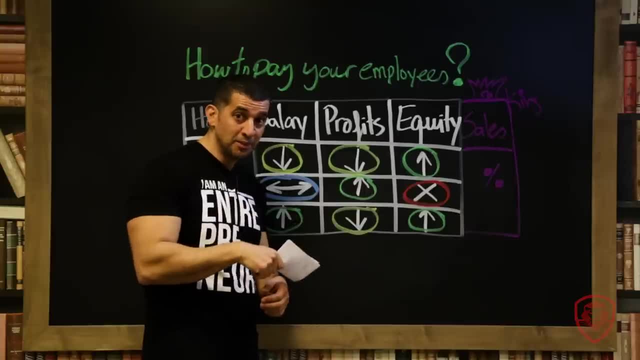 rock star. So you've got to kind of participate. And Jerry Buss eventually gave Magic 5% of the Lakers and put him as the VP of operations, just vice president afterwards. some kind of role he played And so he got equity. Why? Because Jerry Buss locked in Magic Johnson. Magic Johnson only played for one NBA team, was the Lakers Right. Sometimes you've got to lock in a Kobe Bryant, Sometimes you've got to lock in your players In the NFL. they call it. what do they call it? What do they call it? They'll give the franchise tag. So a lot of times quarterbacks will get franchise tag. You can't leave them or trade or all that, so the company pretty much has you. It's like saying a non-compete that you can't leave and go to another team. 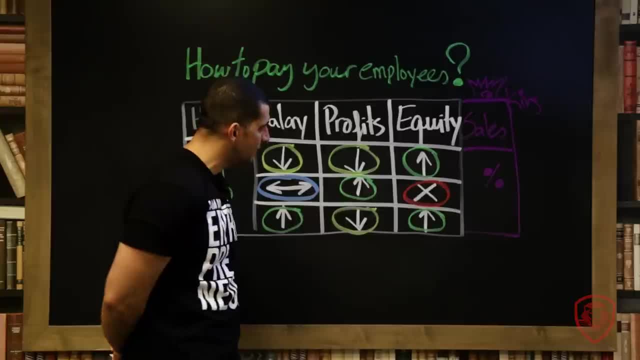 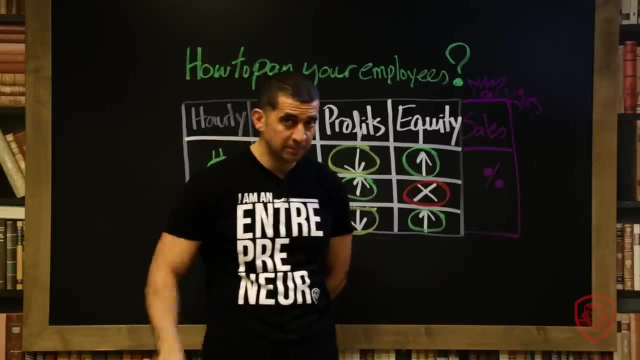 Great. So why would you consider at a point of doing salary and equity at the same time, in both high numbers? Because that talent may be a solid talent that's coming on board Now. keep this in mind: I had somebody that I brought on board that had very, very strong talent, but I had a 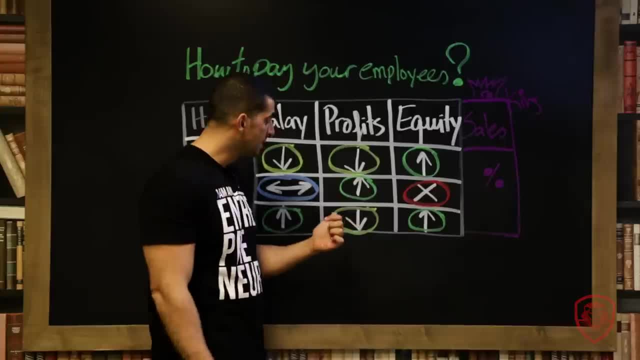 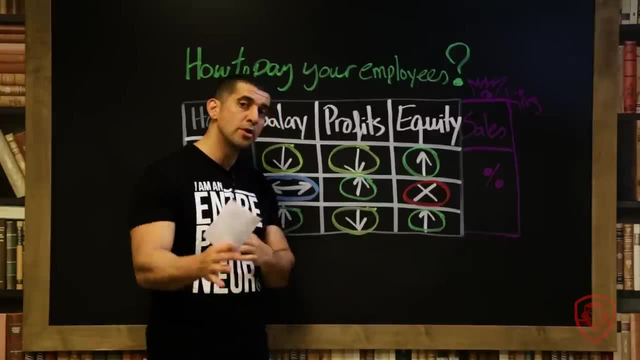 very serious conversation. I said: look, I can't afford a high salary, I can't even afford to give you profits right now this year, but I'll give you a long-term opportunity here. And I wanted to kind of read the person. and the person agreed: 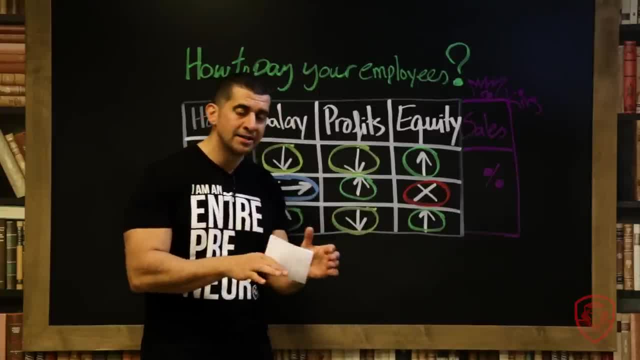 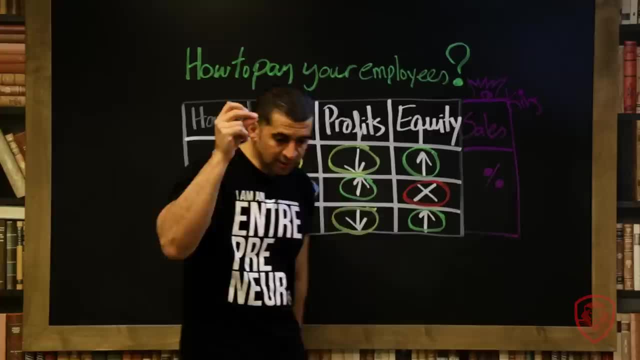 And they came on board And then from there on, the simple question you've got to ask: is this person? how much value did they increase of the company? Think about it. So the moment LeBron James went to the Cleveland Cavaliers, the sports franchise went up $300. 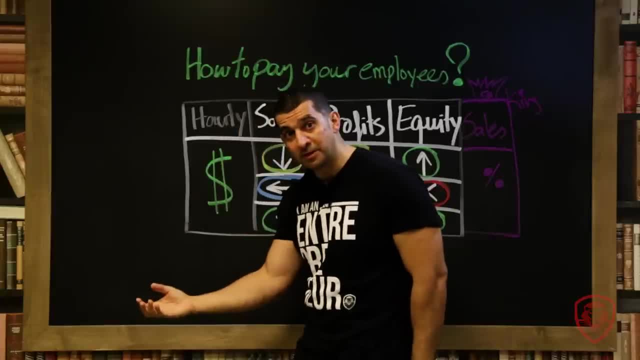 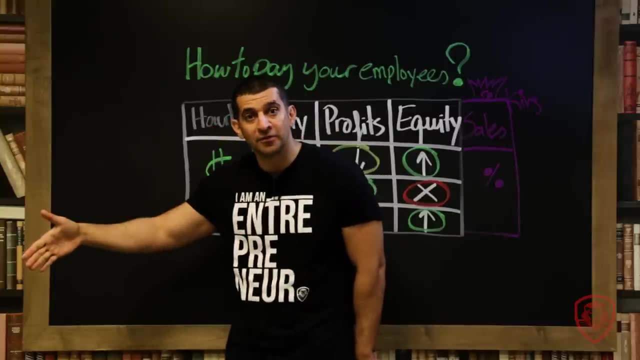 million. So you're paying LeBron $30 million a year. LeBron increased the value of your team by $300 million. Was it worth it? Think about that for a moment. The moment LeBron left Cleveland the first time, they lost $300 million in value. 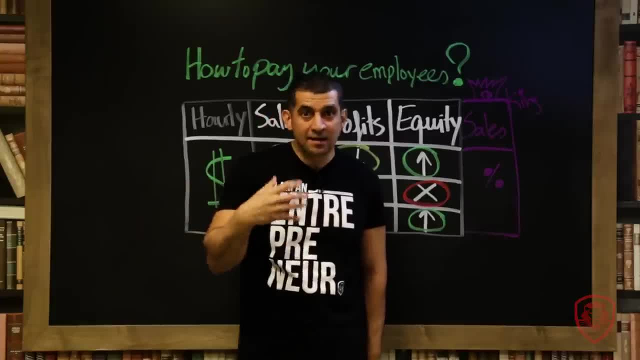 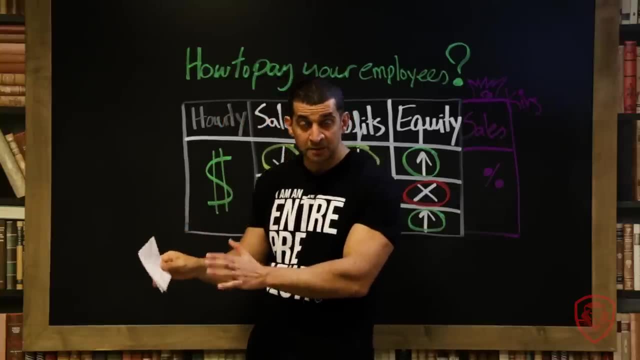 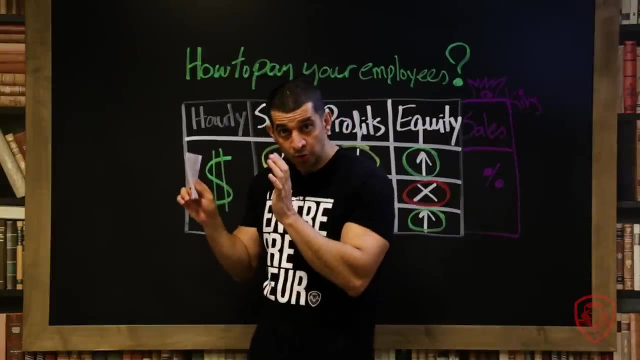 So this is numbers. When I come, I'm bringing value to you. So sometimes in a marketplace, when Sheryl Sandberg's on the market and she's a free agent and Mark Zuckerberg wants her, he brings Sheryl Sandberg to handle the opportunity. 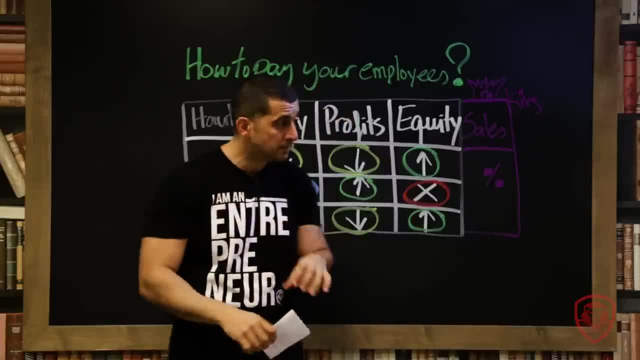 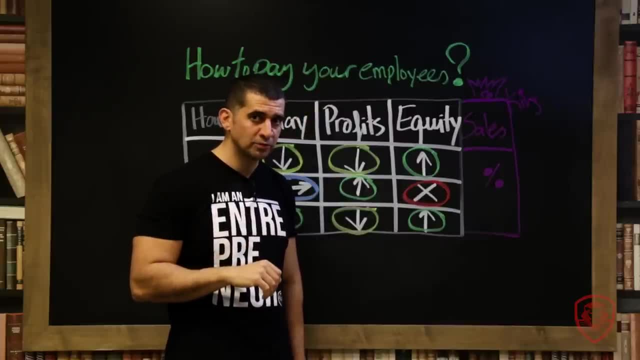 The operations side, the COO, to start making money and all this other stuff for him, Sheryl Sandberg, today's worth $1.5 billion. Do you know what her salary was? Can you take a while and guess what her salary was when she first came to Facebook? I bet you won't get it right. It's not $10 million, It's not $5 million, It's not a million, It's not a half a million. Her first salary was $300,000.. $300,000.. But she got stocks- $30 million. So I want equity, I want to be able to take this company to the next level She did. She turned it into $1.5 billion. whatever the number is now Right. Why? 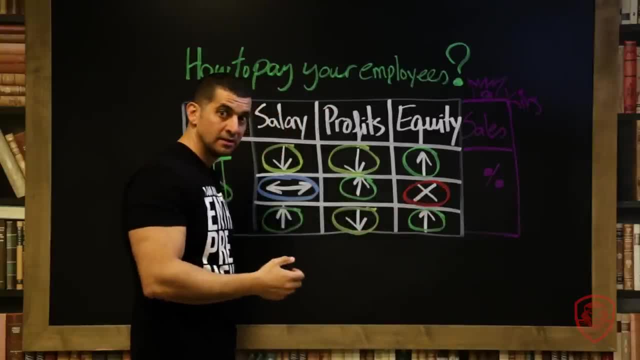 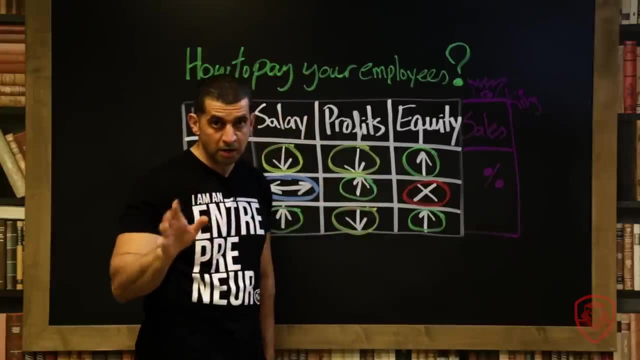 Because she understood: I don't care about salary, I don't care about profits, I'm going for the big play. So you're realizing sometimes in a market you have some talent that you've got to work that out with. Now, for the most part most companies don't give salespeople equity. 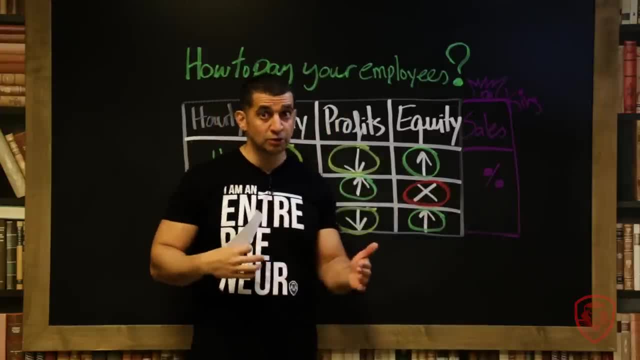 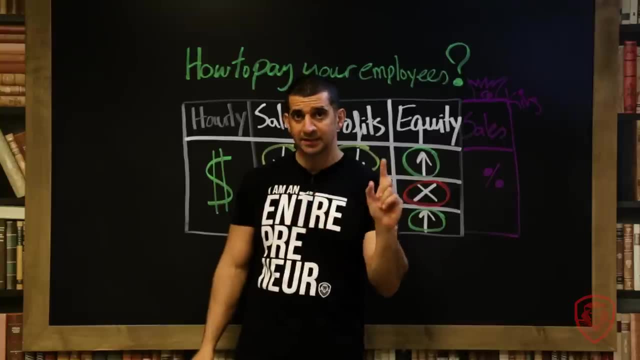 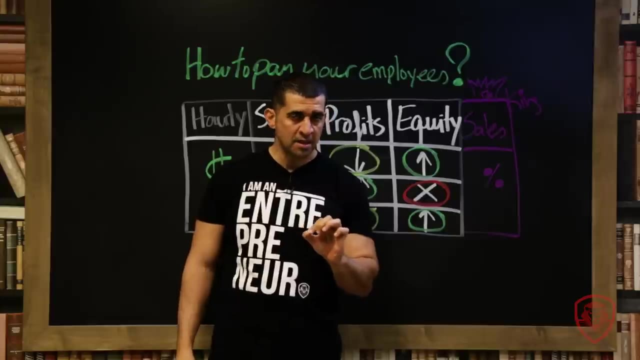 I like to do it. I like to do it And we have a certain program that we do for that. Why? Because I think sales a great sales manager or sales leader. let me restate that, not necessarily sales manager. A great sales leader is very hard to find. 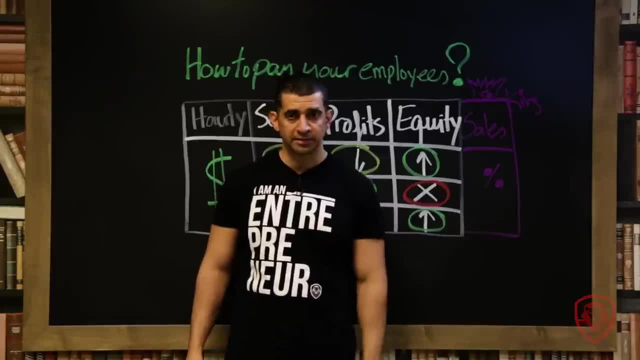 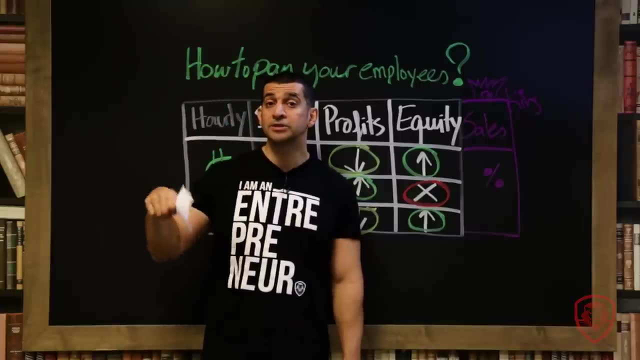 Very, very hard to find And you've got to value your sales leaders. You've got to value your great sales leaders, Got to value them. A salesperson can come and go a sales leader. they know how to teach other people how to. 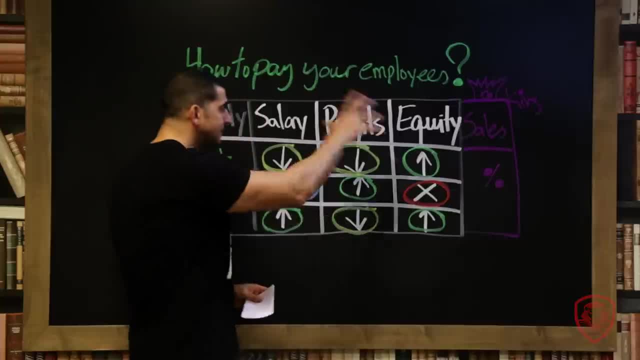 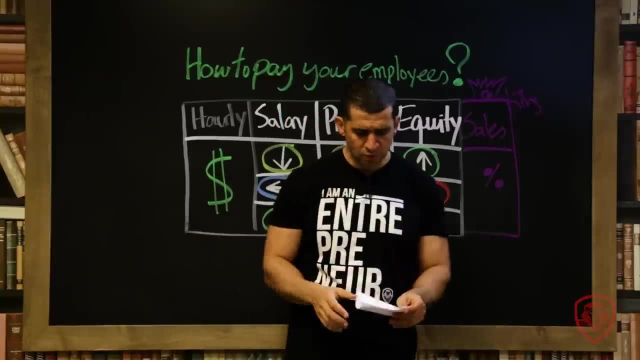 become sales leaders themselves. Very difficult to find that. So this is an idea for you to be thinking about when you're hiring somebody: How do I combine what? And, by the way, a lot of times when you're looking at this. I'll go into my last points. 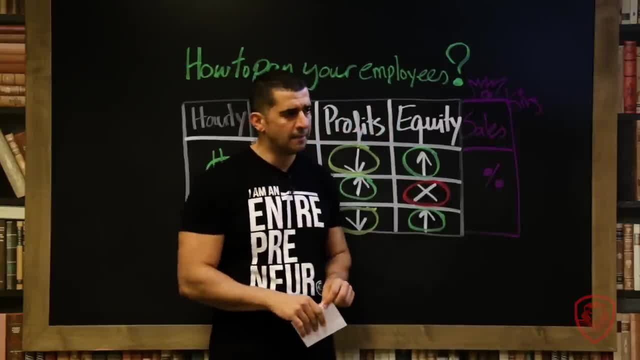 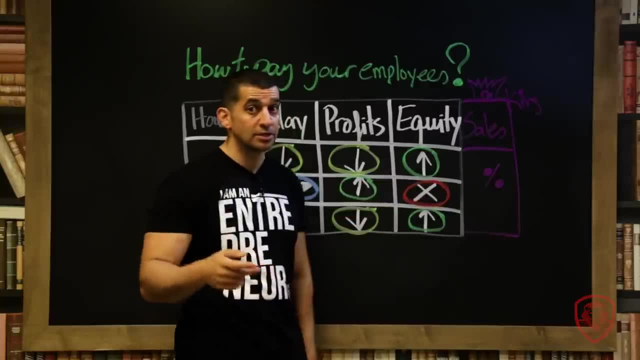 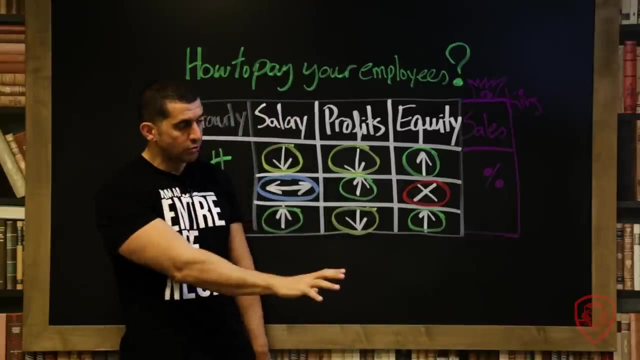 here with you. A lot of times when you're going into this, you've got to know your own numbers. For instance, if I'm giving equity to somebody, I'm giving equity to somebody who is irreplaceable. If you're watching this yourself and you are on the hiring end, so you're the employer. 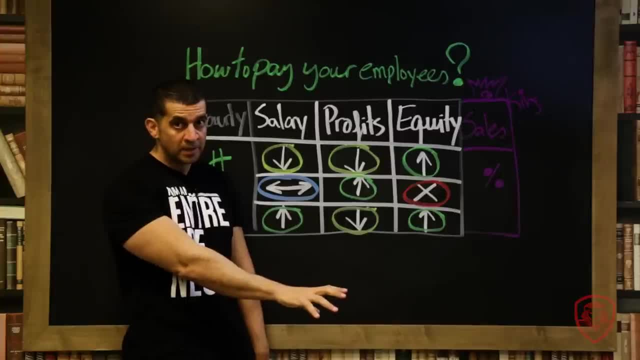 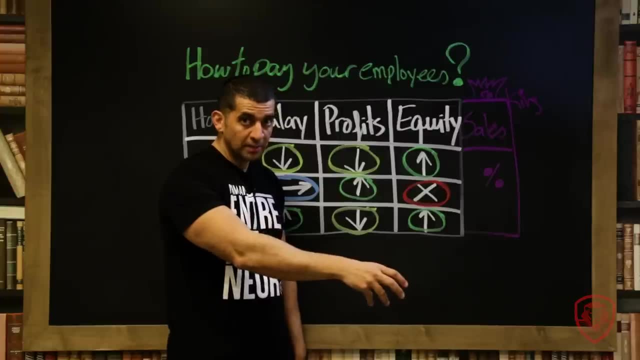 you're thinking about hiring an employer or promotion or hourly or equity, or an executive or salesperson, you've got to ask yourself: is this person irreplaceable? So what is irreplaceable? They have certain relationships that you need, Okay. 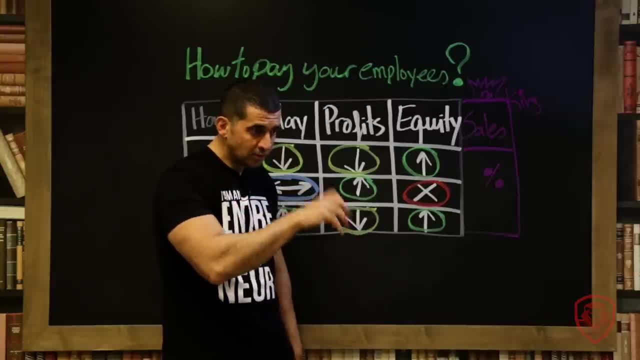 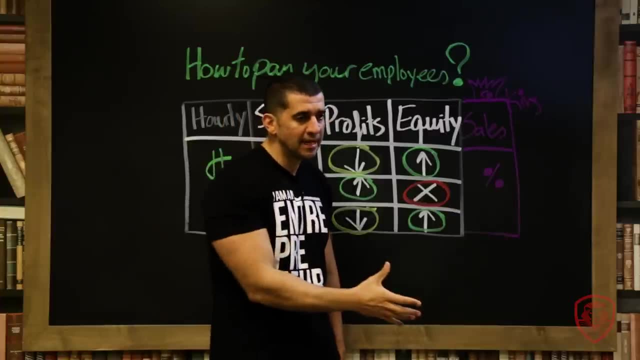 There are certain contacts that you need them to be with you long term. There are certain skill sets that they have that you need them to be here. There are certain capital they're bringing to the table. that's a non-measurable capital, It's not necessarily money, but they increase the value of the company. 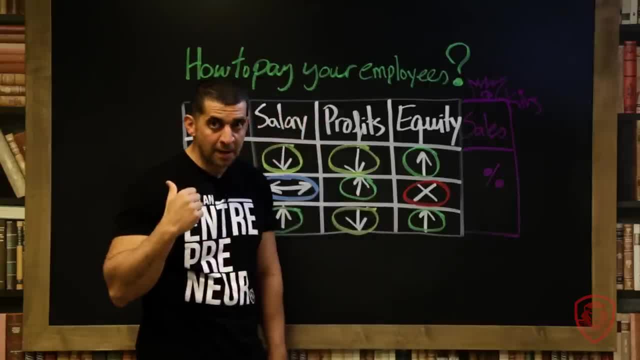 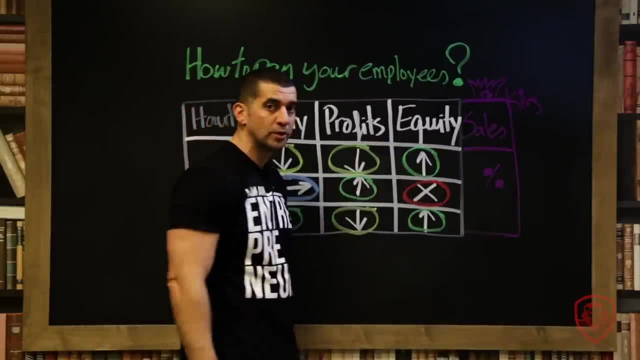 You need to understand that person's irreplaceable. If you're on the complete opposite end and you're maybe an hourly or salary and you kind of are wondering what is your edge going to be when you're asking for profits or equity, 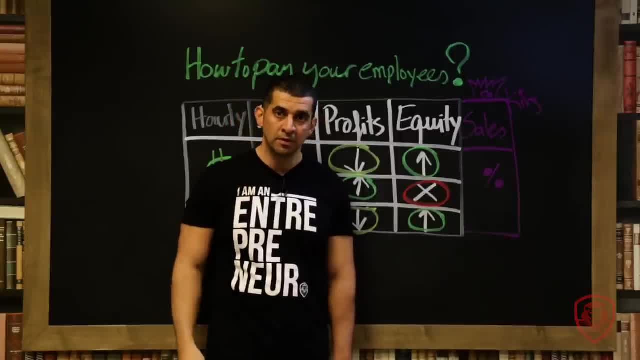 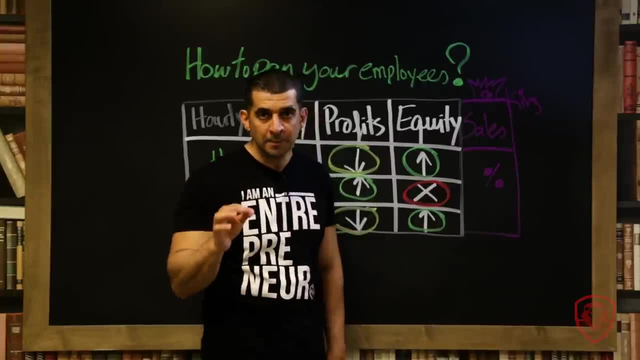 well, you've got to ask yourself the question: are you irreplaceable? Because if you're irreplaceable, then it's very easy Value can be determined. if you're irreplaceable, If you're replaceable, what do you want to have? 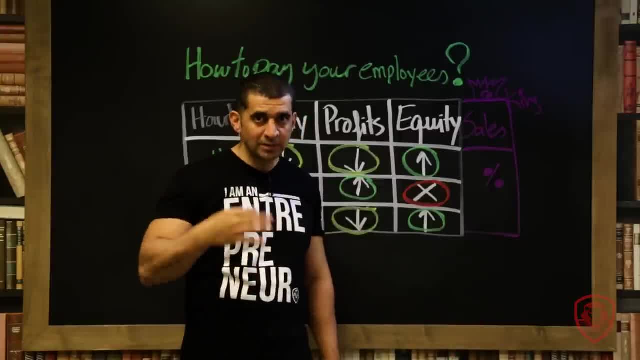 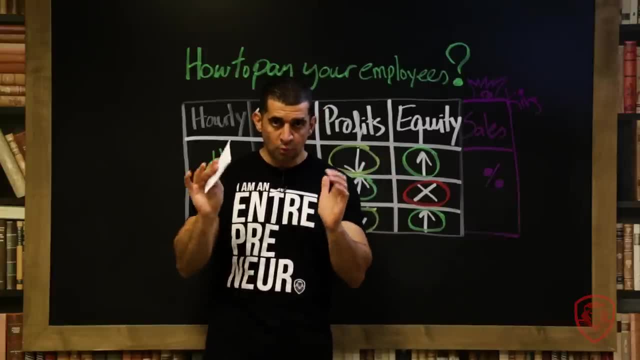 You have no leverage, So you've got to make sure you're replaceable. I literally sit down with my team and I tell them: you need to become irreplaceable and you'll increase the value you have with me, with the companies, long term, with us working. 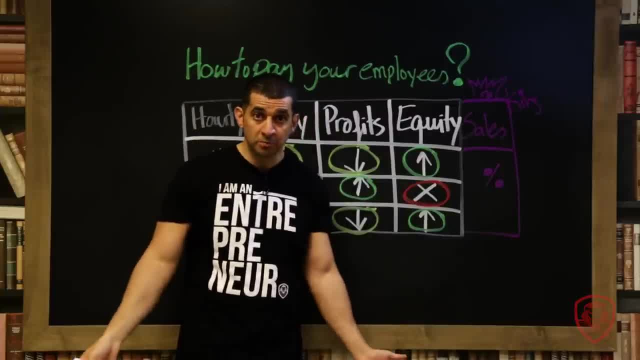 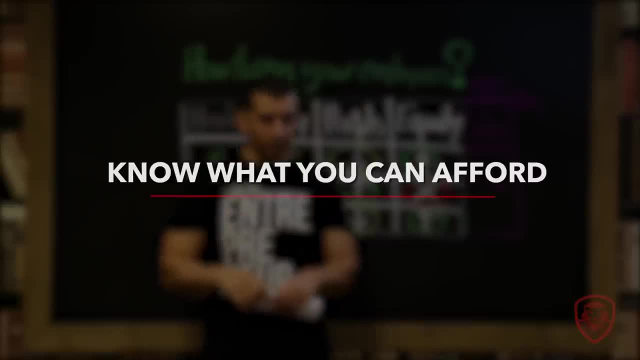 together. If you're not a replaceable, what are we doing here? What are we doing here? You've got to be replaceable, right, Okay? So now strategies. Strategies to be thinking about. Number one: Know what you can afford. 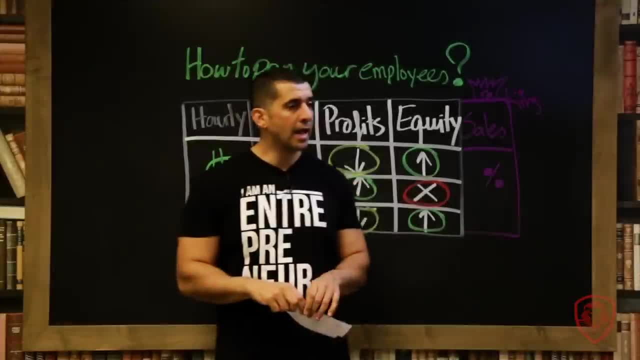 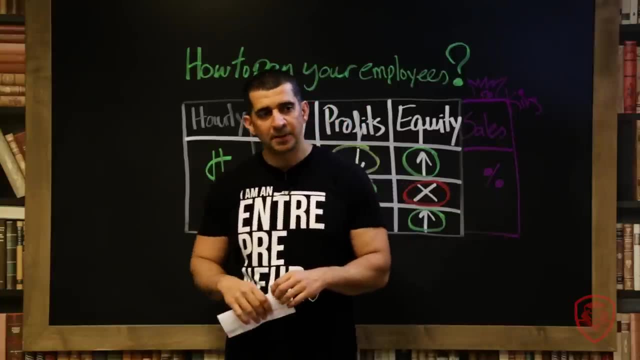 I had a guy ask me the other day: Pat, there's this person I want to hire and man, he's so great, I love him, but he's got kids, he's got a wife and his last company- they paid him. 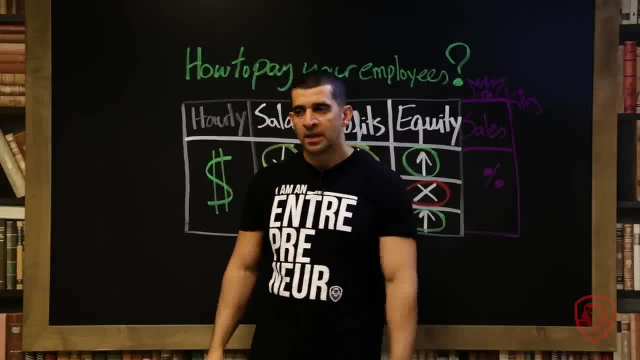 $180 a year, but I know we've got a great opportunity. I want to bring him on board, And his last company was a part of it. When they were bought, he made a half a million dollars and he's coming to me. 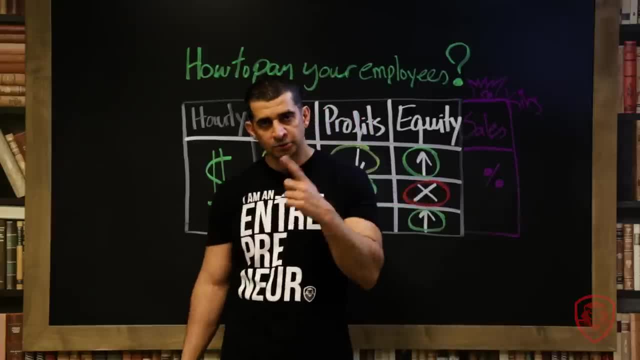 He would completely change the life of the company if he came on board. That's okay. How much did your company make last year? Well, we grossed $1 million. Okay, what did you net last year? $50,000. 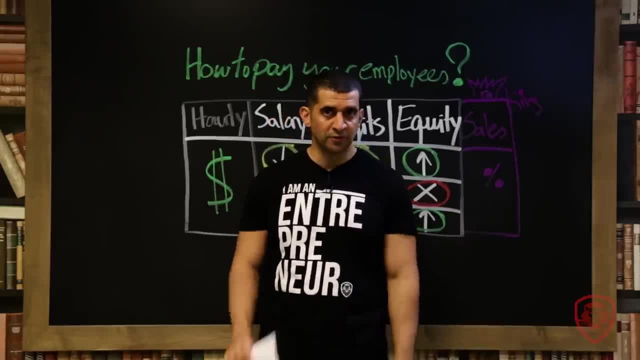 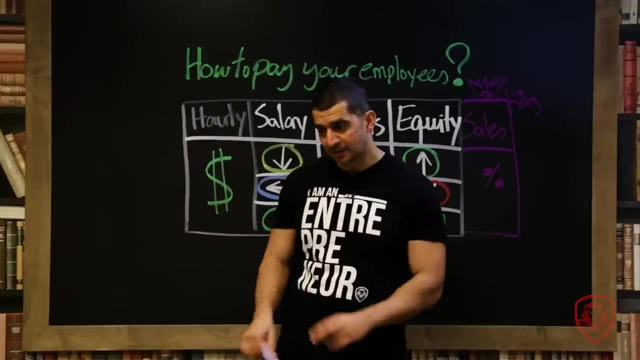 I said: so what can you afford to pay this guy? I can afford $50,000.. I said: you can afford $50,000?? I said: what else can you give him? That's it. I said: what is your projectory of your company? 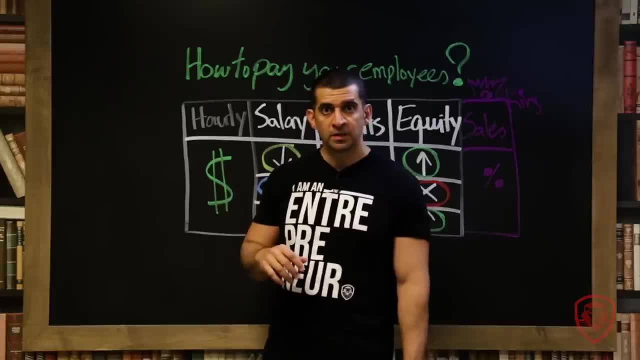 Like: did you go from $100,000 to half a million to a million? No, What was the projectory? It was a slow project. I said: so have you guys been going like this? No, we've been going kind of like this. 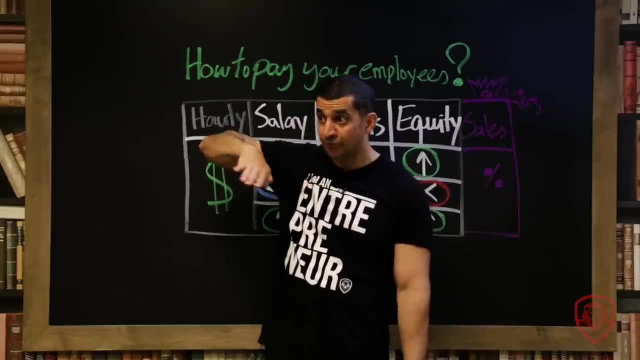 You know that's not a person to come and say: oh, they're going from $100,000, half a million, a million, $2 million, $10 million, $40 million. This is great, right? I want a piece of this. 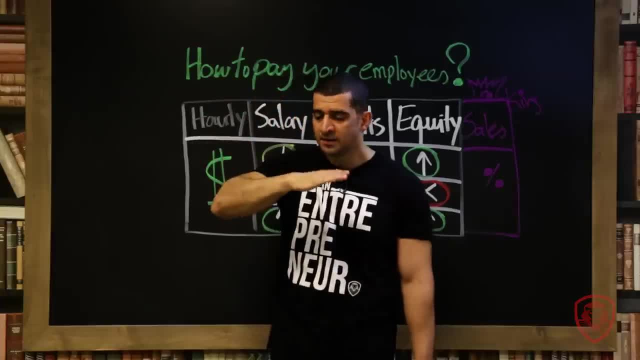 In three years my buyout's going to be $4 million. I'm interested, right, But if it's like this, you don't have an argument to give that guy the talent. He's going to come and say: what are you talking about? 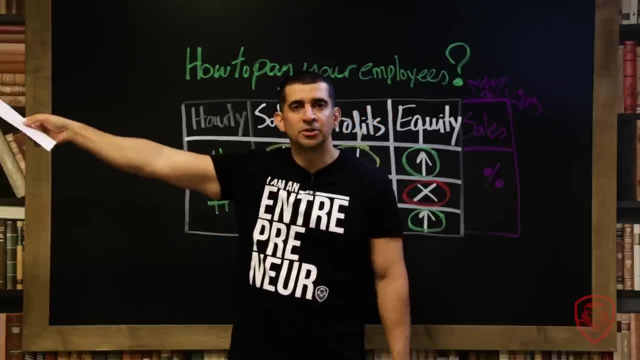 And you can't give him $50,000, while his expenses he's 36,, 37 years old, he's got a wife and kids and a mortgage. he's not going to do it at $50,000.. So you need to know your numbers. 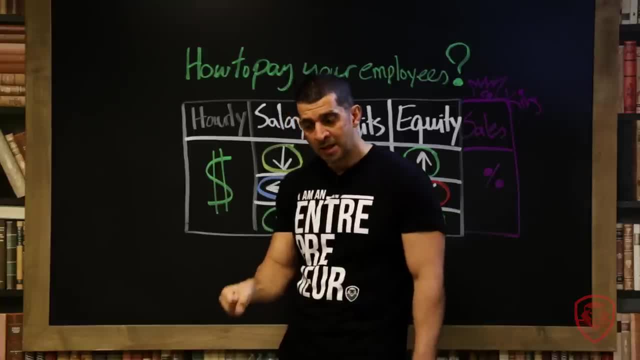 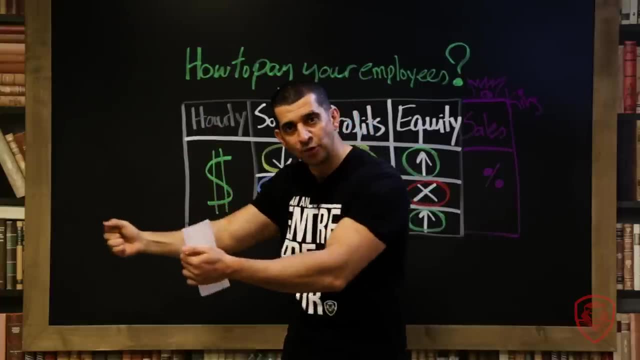 You may bring him in on your advisory board and have him stick around on the advisory board And you work your tail off so he sees the projector and then you say, hey, you want to come and be the president Now. I can afford $150,000.. 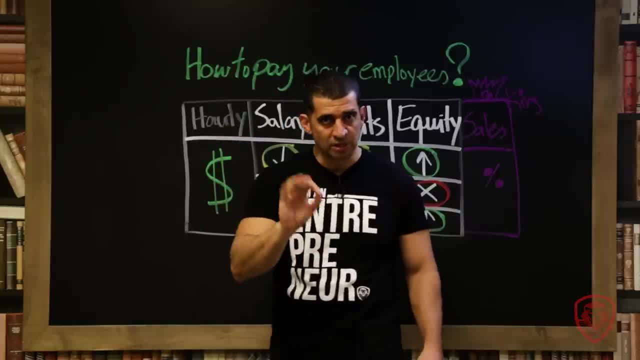 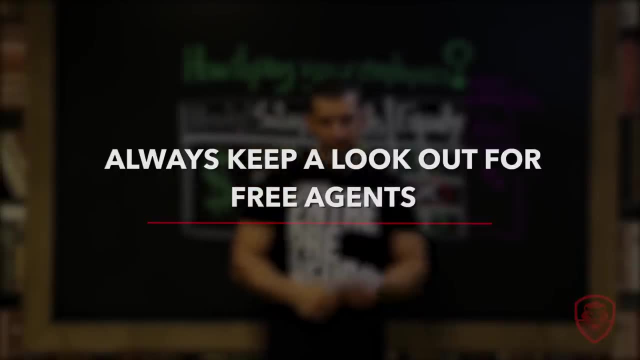 I'm coming in because he's falling in love with the company now Make sense. So that's a completely different story. But you need to know your numbers. Two: always keep a lookout for free agents, Always, Always keep a lookout for free agents. 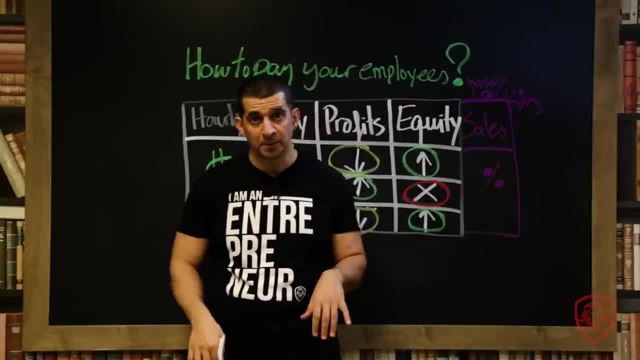 We've got the insurance convention coming up next week. I've got so many messages from people telling me: Pat, you know what can I do to be part of a VP with your company? I want to work from the home office side. 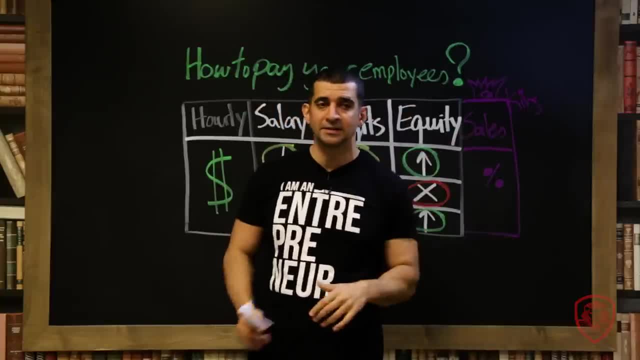 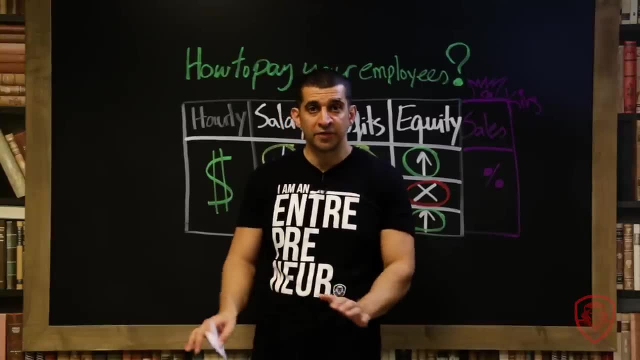 I think I can bring value to your marketing side, Your operations side, All this other stuff. I'm always looking for free agents. I'm always looking for great free agents. I mean amazing free agents. Why? Because free agents, it's free agents. 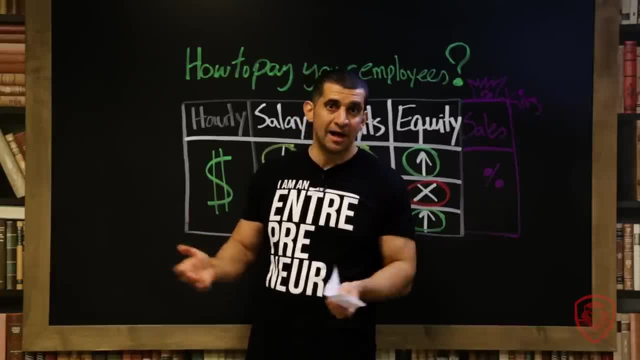 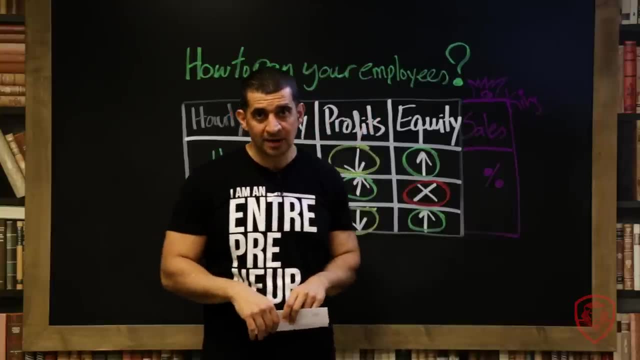 You know, when LeBron is on the trading blocks, you've got to pick him up. This doesn't happen all the time. When you get some killers on the trading blocks, you've got to make sure you go pick those guys up. So always keep a lookout for free agents in the marketplace. 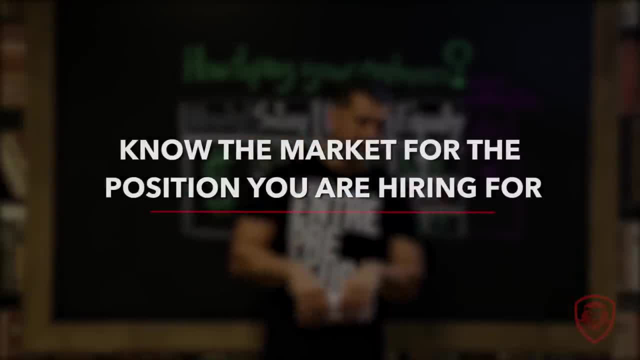 Number three: Know the market for the position you're hiring for. For instance, I had somebody that came to me and said: well, Patrick, you know, I want to one day make $300,000 a year with you. I love this guy. 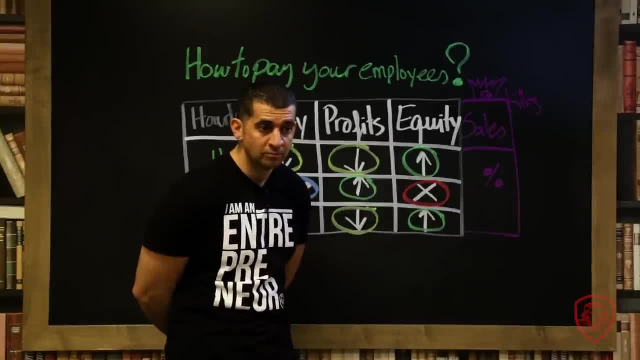 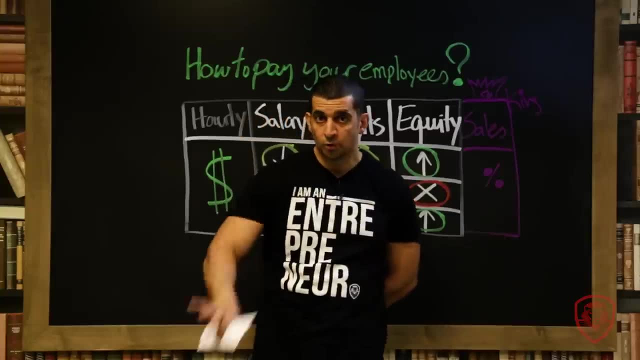 I said really. He said yes. I said that'll never happen. Why not? Because the market for what you're doing is this. Oh well, I'm going to go somewhere else. I said, no problem, Take the next two months and you start looking. 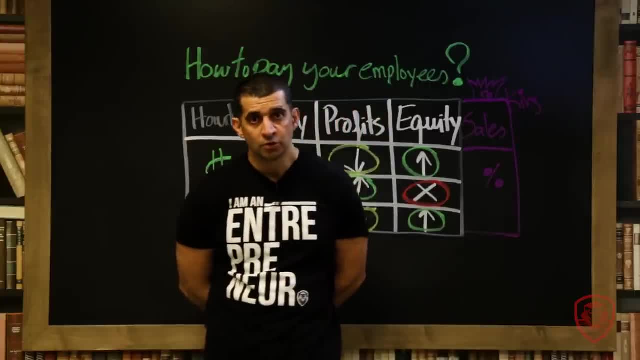 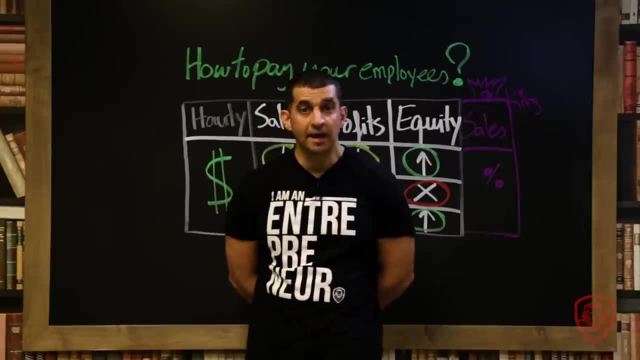 This is not today, This is years ago. Take the next, you know, two months, and start looking And he goes looking And he comes back and I said: so what happened? Well, I got a lot of offers- Great. 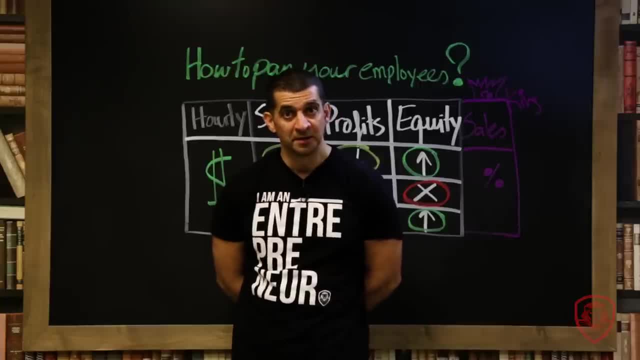 Did anybody offer you $300,000? No, Oh really Yes. So what's the number? Well, you know what my number is. I said I know the number for your position And I just took the printout. 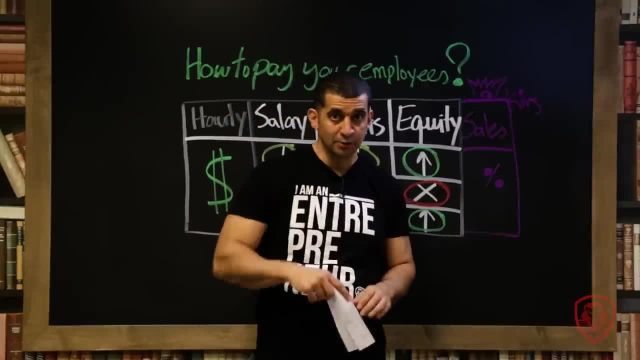 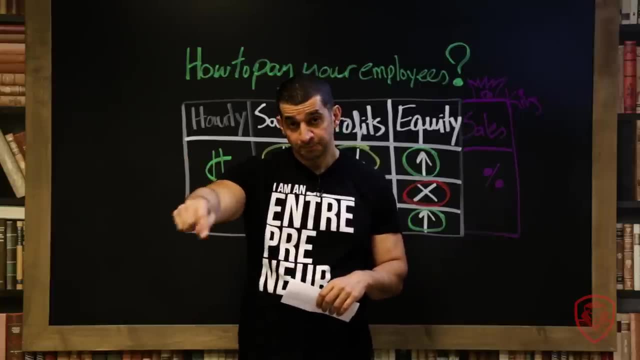 This is your number. This is exactly your number. This is exactly your number. Stuttering, stuttering, stuttering. Did you talk to other people? Yes, This is your number. I'm willing to pay you this, which is more than this. 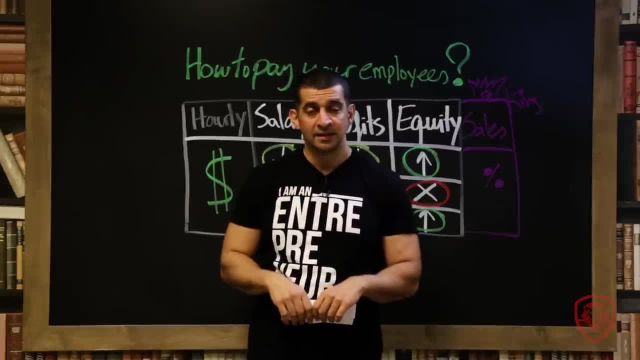 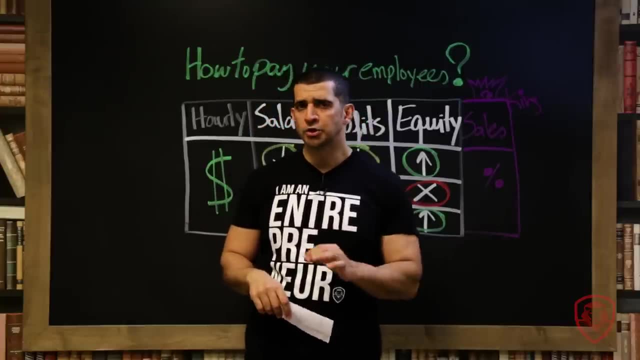 You'll be the highest paid person at this position, but this is your number for this. And he says, oh, okay, great, All this small conversation, everything was done with, and we've not had a single issue ever since then. 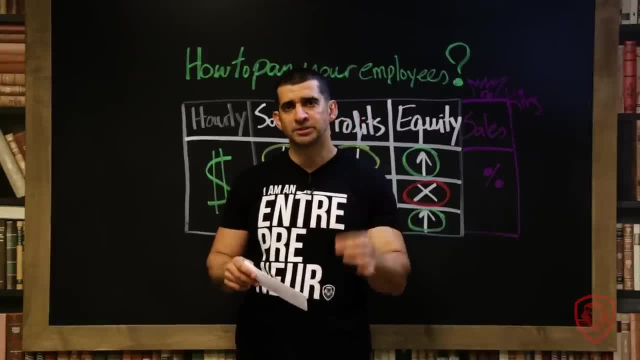 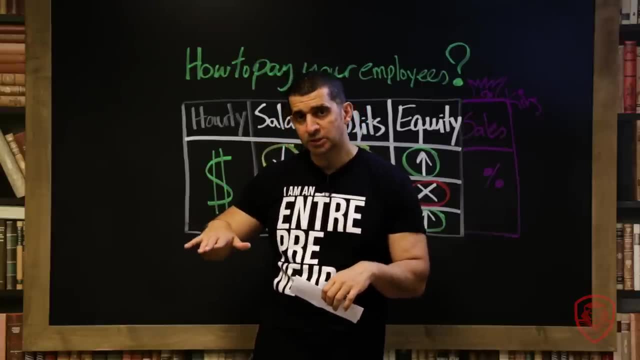 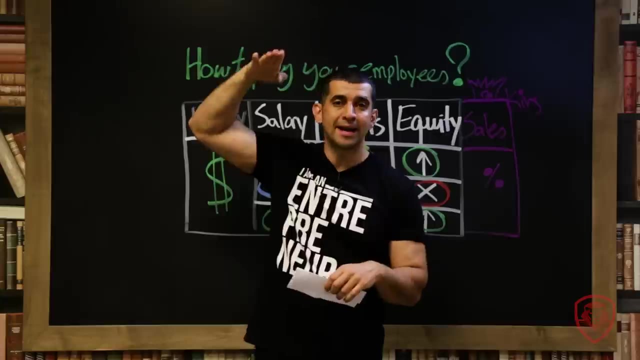 So you need to know what the market value for the position you're hiring. for the regular person, the low skill level, not as much expertise, and the big shot guy, the market value is going to be higher for this person, but it's still not dramatic of a difference we're talking. 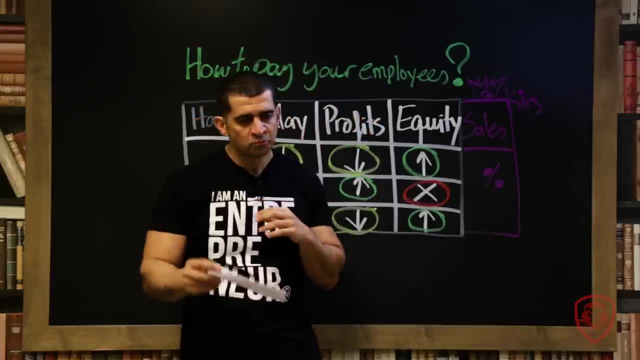 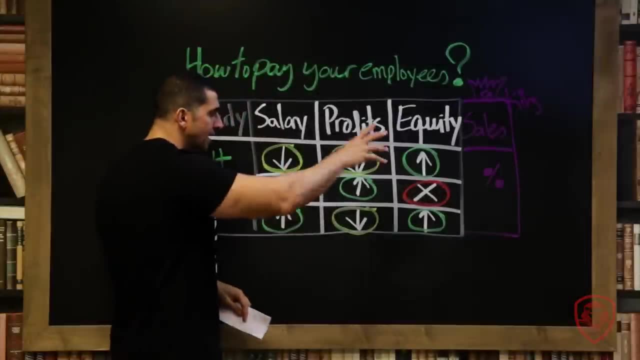 about. So study your market value for any position you're hiring for. Sixth, be willing to customize pay depending on talent. This whole thing is: you're going to get judged based on your creativity, on what you can do when you bring some talent on board. 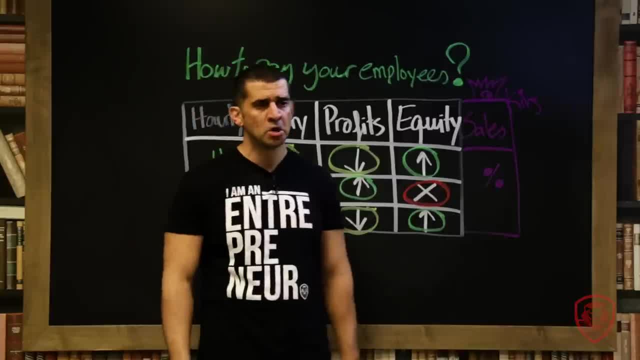 And I'm not talking about sales. I get a lot of sales people that'll come inside and they'll say to me: well, Patrick, let me tell you when I'm coming on board, you've got to do this, this, this, this, this for. 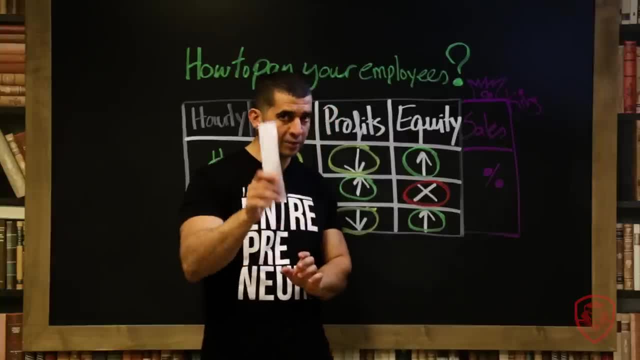 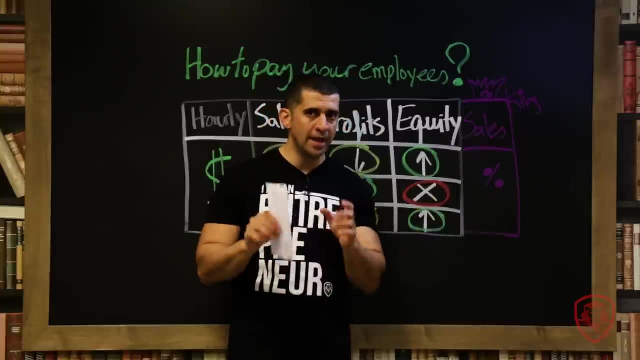 me because I'm this, this Great. I rarely, rarely- do that with anybody that comes from the outside, And why? Here's why: Why: Because the people who end up becoming your best sales people are the ones that came in not asking for anything homegrown. 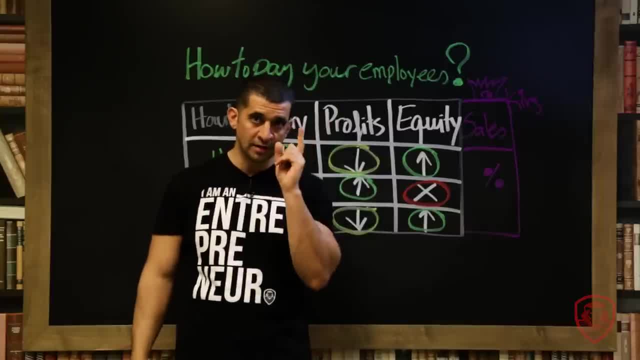 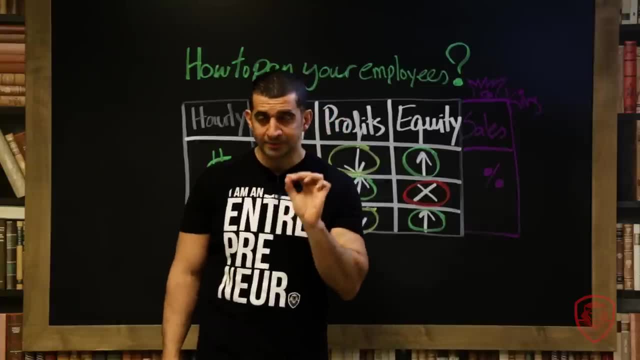 They grew. You better make sure you take care of those guys, Because if you don't, I will. I'm just telling you right now, Somebody else in the marketplace would be more than glad for that person. If they're the loyal, talented people that want to work hard, they just want a company. 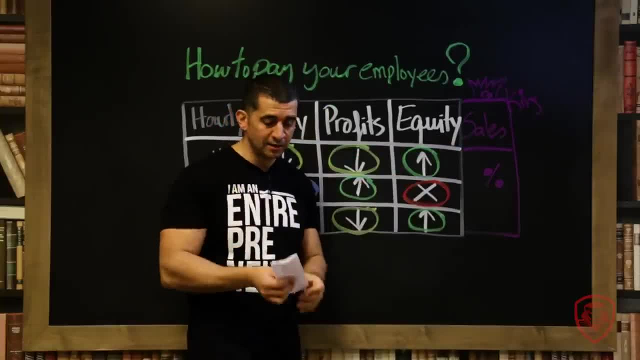 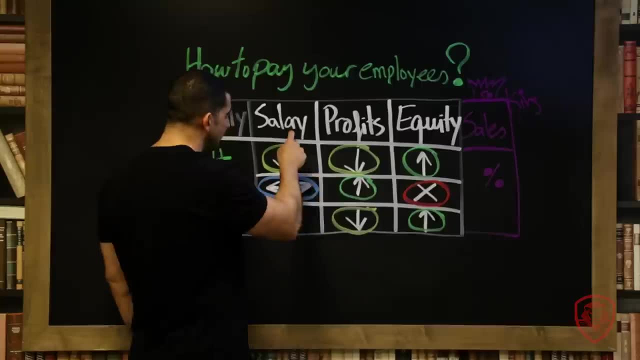 that takes care of them. You don't take care of your best sales people. somebody else will. Okay, But learn how to customize it. Just try it out, You know what. Take this whole thing yourself, Take your paper and tell yourself you know what. 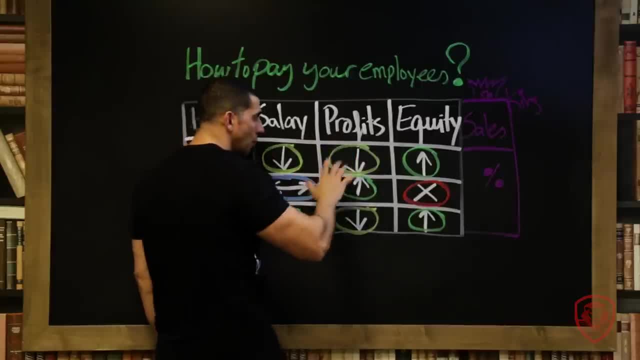 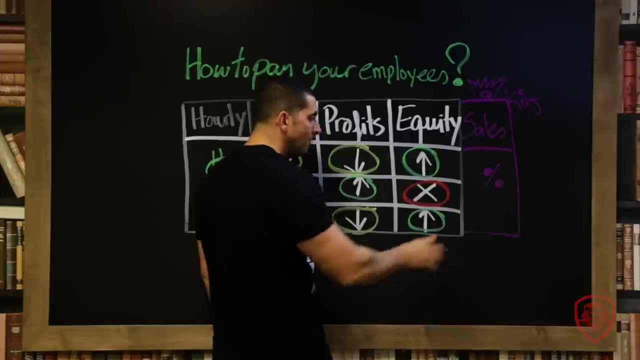 If I did this and I did this and I did that. What if I give them bonus and I give this? What if this guy's a salesperson? Let me see what I can do with my compensation plan to do it this way. What if I did something with our sales guys and they were able to participate in that? 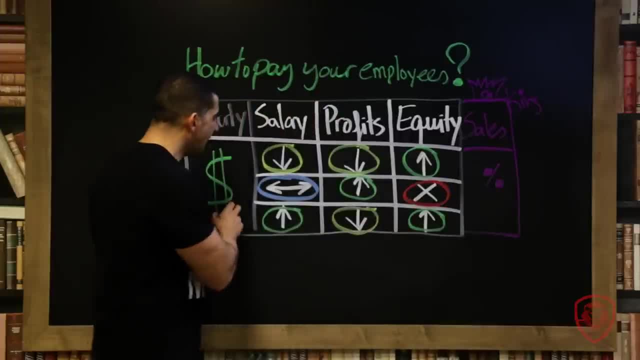 What if I did something with my sales guys and we participated a little bit in the bonus? What if I got my hourly guys and figured out who it is and got rid of some and increased some of them and told them what they need to do? 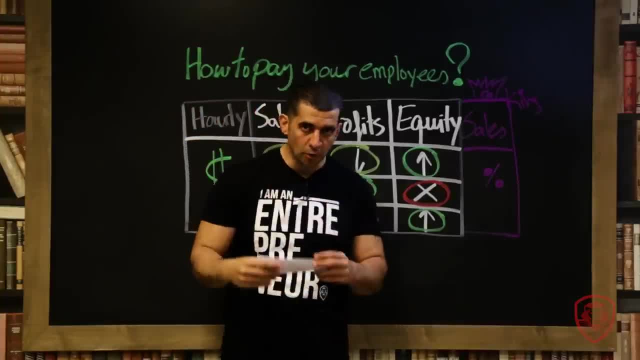 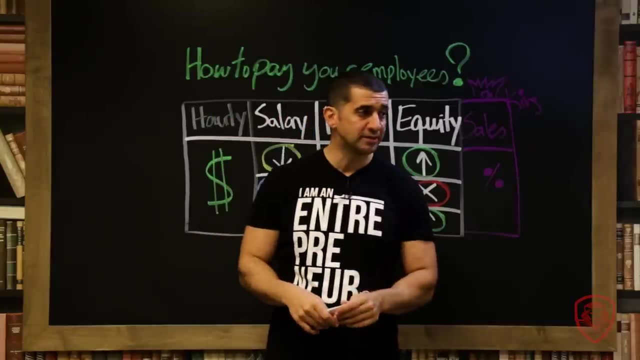 Just play with this. This is very fun. This is great Because it also you're putting a game plan for yourself on how to get people advancing and how to get talent to your place. Yeah, And then, last but not least, which is very simple, set up a comp plan that incentivizes. 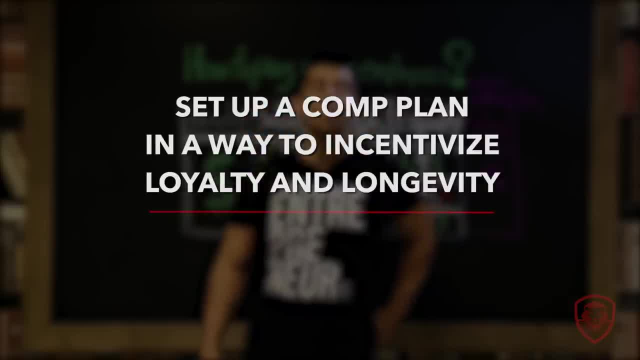 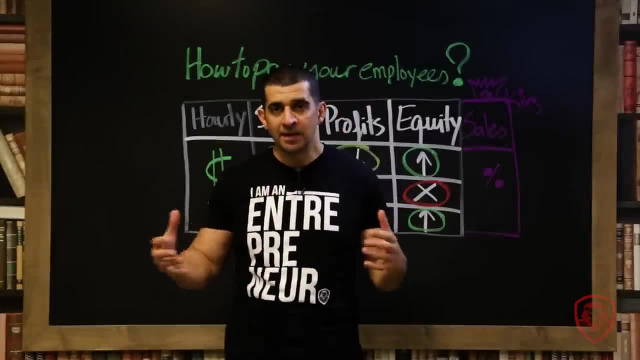 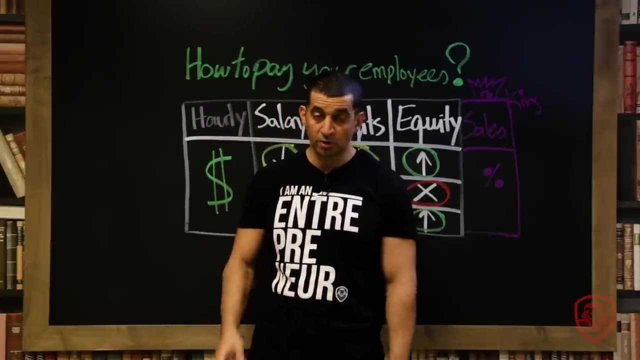 and motivates people to be loyal to you and motivates people to increase their longevity with you, if that makes any sense. Depending on how you set up your pay structures, you're going to get my loyalty and you're going to get my determination to stay with you long term. 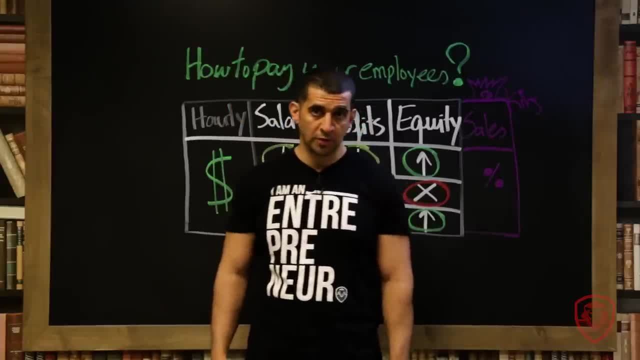 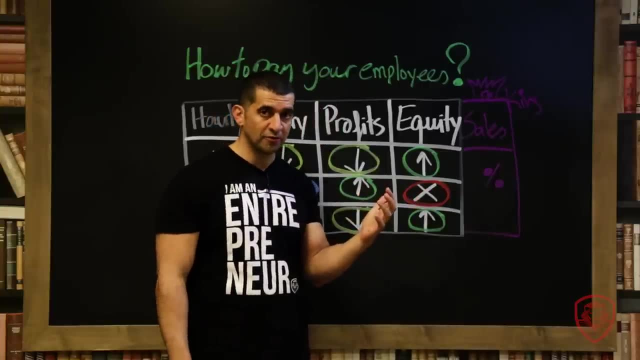 It's the first thing I told you when I opened this video up. I talked about that with you. So if you do that and you're giving me equity and maybe there's a five year vesting period for me to stick around for five years, but five years later I'm going to participate. 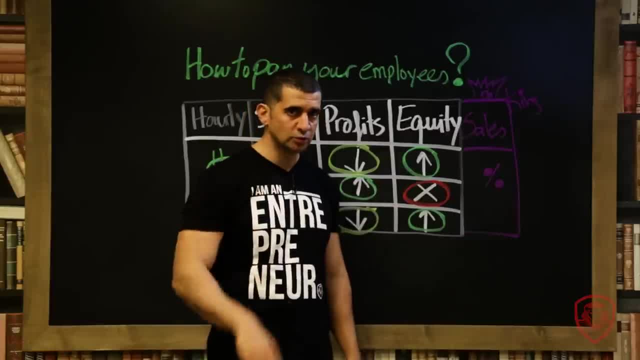 in dot, dot dot. you're getting me to realize and say I'm going to be in business with you long term And at the same time you'll also realize which one of the people you have in your company are long term people. 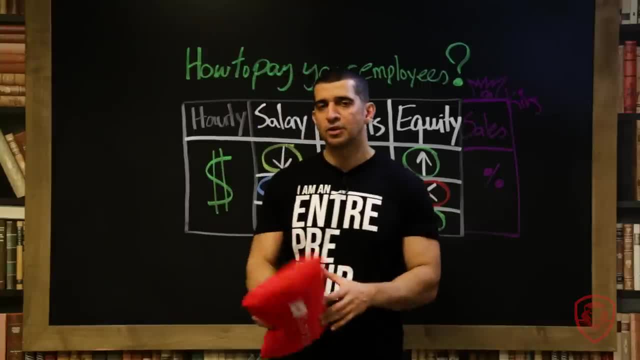 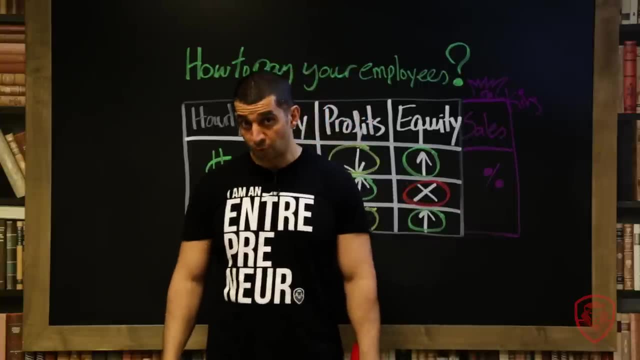 Anyways, with that being said, so this again. I told you this is not going to be a very, very exciting topic, but it is a topic that many of you that run multimillion dollar businesses ask me about regularly, And I know that you're having challenges with this. so you can post any comments or